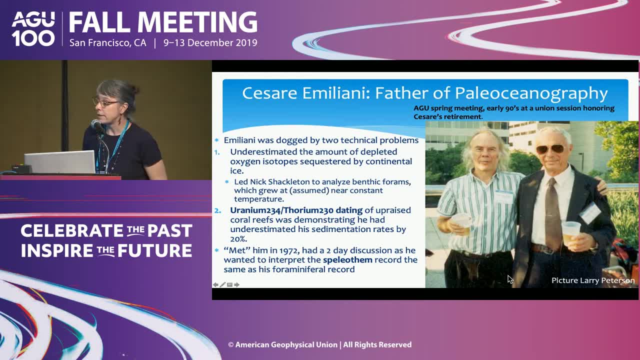 and what his influence was on your career. So it turns out I did meet him. There was a two-day discussion on the interpretation of speleothems back in 1972. My father did most of the talking because I was about six months old at the time. 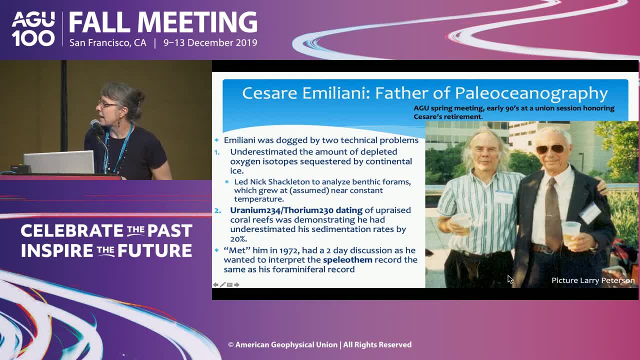 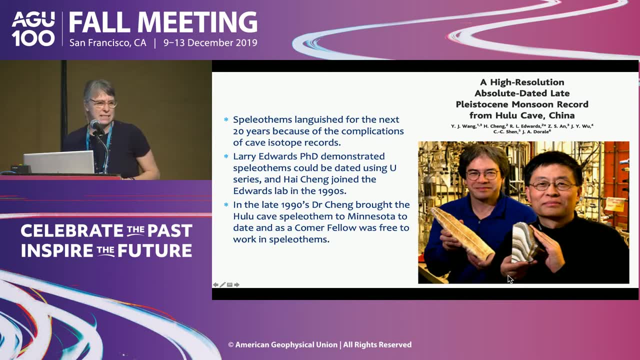 But there is a connection. But that leads nicely into this lecture, because speleothems languished for about 20 years after that, until development of uranium series dating in caves improved the dating of cave techniques And people really began to understand the systematics. 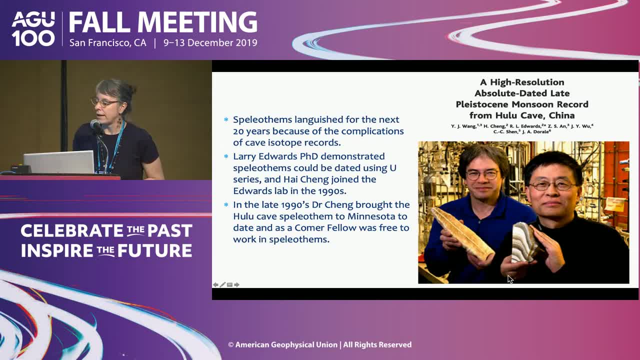 of speleothems. In the late 90s a very special speleothem came to Minnesota And through the Comer Fellows and with work that Hai Cheng did with Larry Edwards, the Hulu cave speleothem was developed. 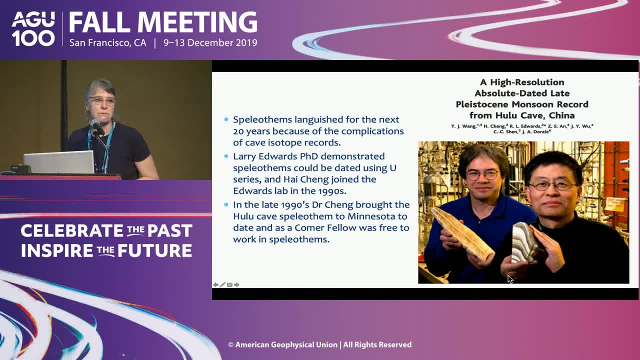 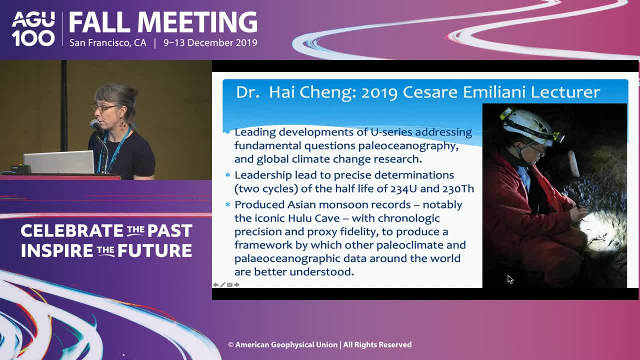 And we're still seeing its influence on our dating and on our understanding of paleoclimate records today. So our Emiliani lecture today is special for leading development. He's been a leader in the development in uranium series dating, addressing some of the fundamental questions. 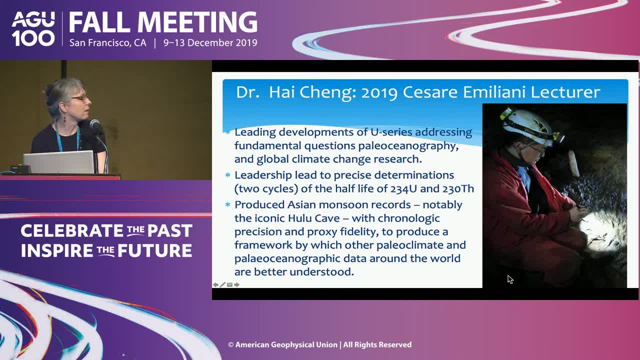 of paleo oceanography and global climate change. He's been a leader in improving the dating techniques, as well as producing some amazing Asian monsoon records, including the iconic Hulu cave record that has improved our paleoclimate data from around the world. 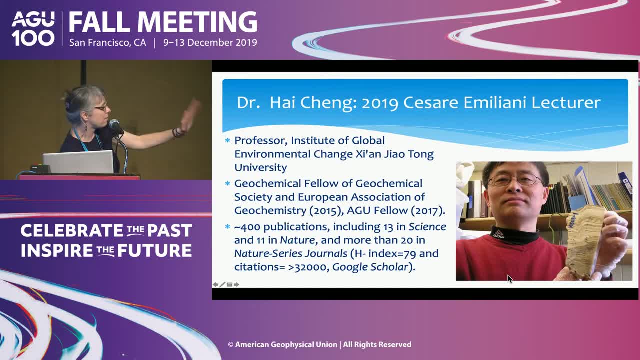 Now I know some people are really into numbers, And so I've got some numbers up here, Publications where they were published: H and X. Everyone loves the H and X And I think you'll agree that Hai Cheng is highly qualified to be our Cesar Emiliani lecturer. 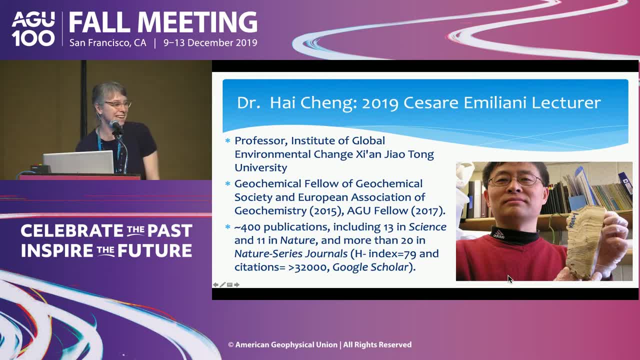 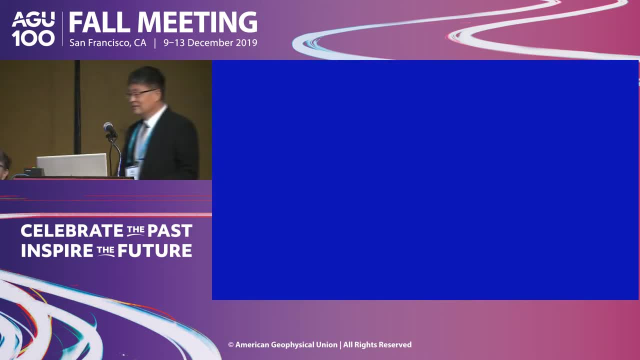 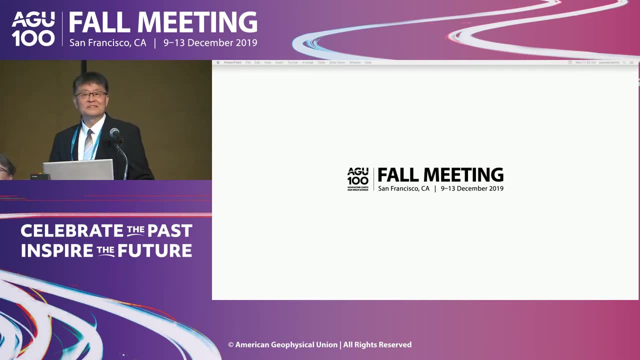 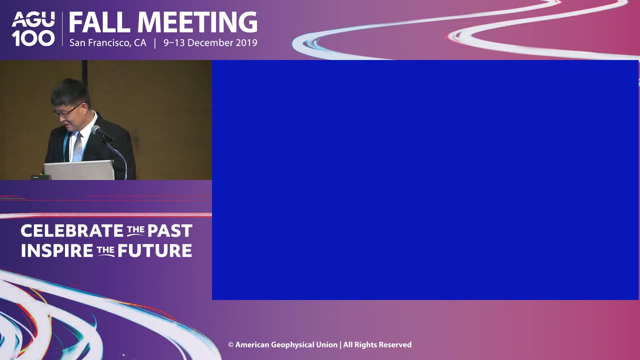 So with that, I would like to welcome to the stage and stop talking and let him tell you about his science. Thank you for your introduction. This is a. It's a great honor for me to give this talk. OK, So probably I might not be able to use this anyway. 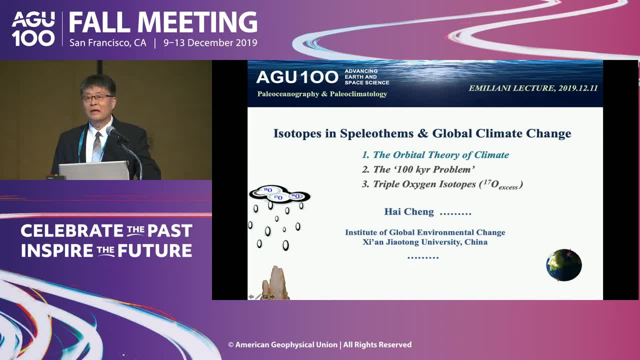 So my topic is isotopes and global climate change. Mainly, I'm going to address some aspect of orbital theory of climate. If I have time, I'm going to talk a little bit about the 100,000 problem. This is a classic problem in this field. 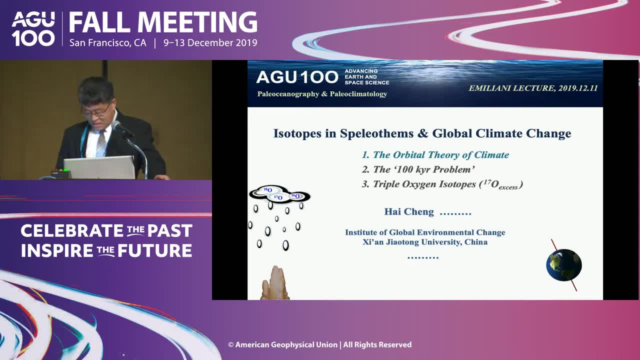 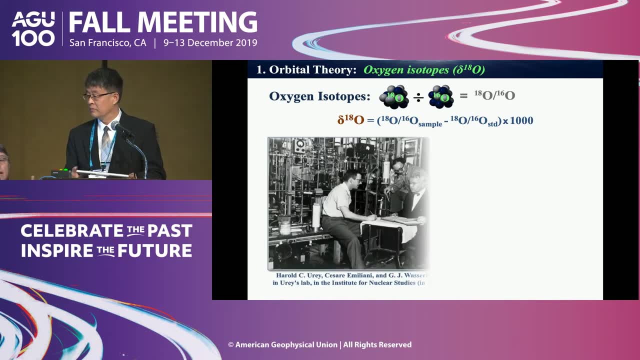 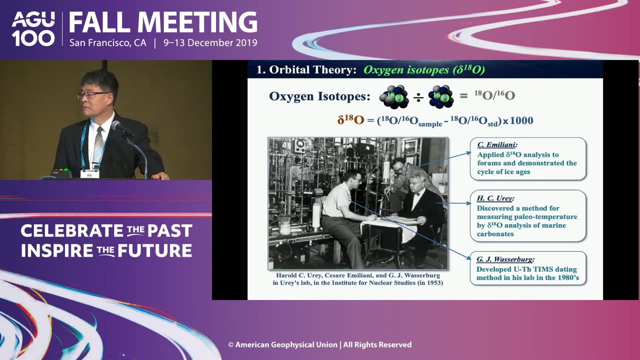 And the triple oxygen isotopes. OK, I don't know if that's OK. Oxygen has three isotopes: 18-0, 16-0, and 17-0 as well. 18-0, 16-0 ratio is commonly used with a delta notation. 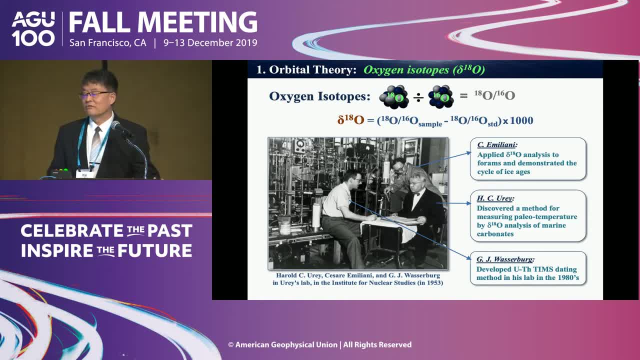 we call data weighting. This is the definition In our field. this picture has three very great scientists. Emeliani applied a data weighting analysis to forums and demonstrated the cycle of ice age. Urey discovered a method for measuring paleo temperature by data weighting analysis of marine carbonates. 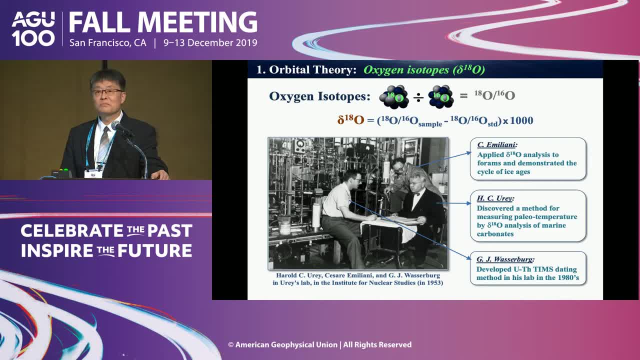 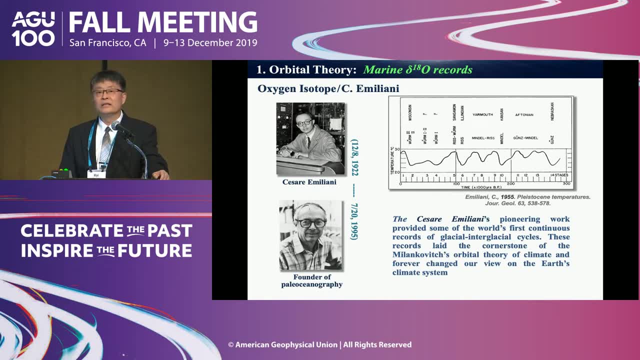 And the Watsonberg. He developed uranium theories- Tim's method- in his lab in 1980s. In 1955, Emeliani published his long record, temperature record based on measurement for data weighting of the forums. His pioneer work provided some of the world's first continuous 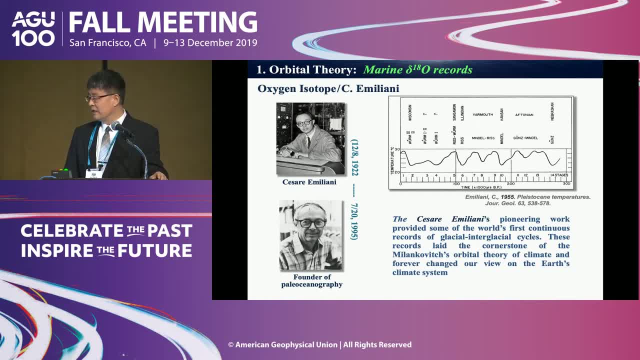 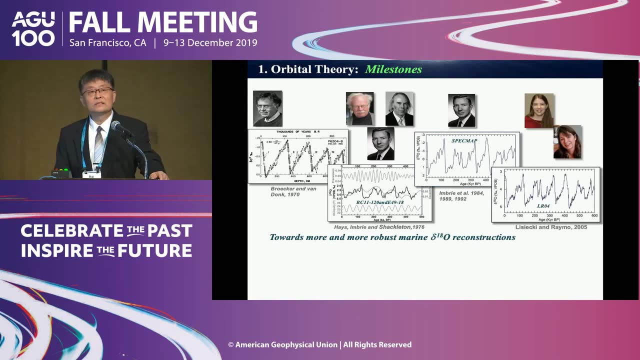 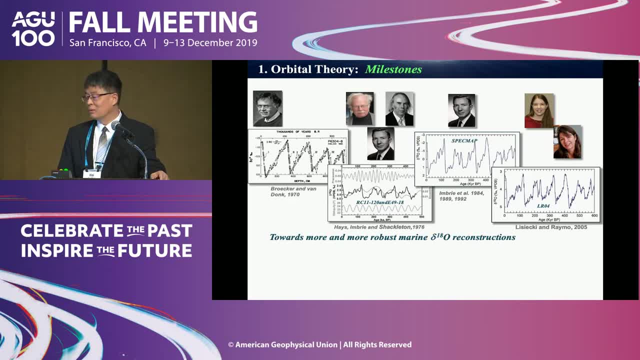 are a bunch of milestone works toward a more and a more robust marine data weighting reconstruction. Notably, however, all the chronologies are still essentially based on the orbital tuning strategy. one of the basic assumptions: phase lag of 5,000 years to some insulation. 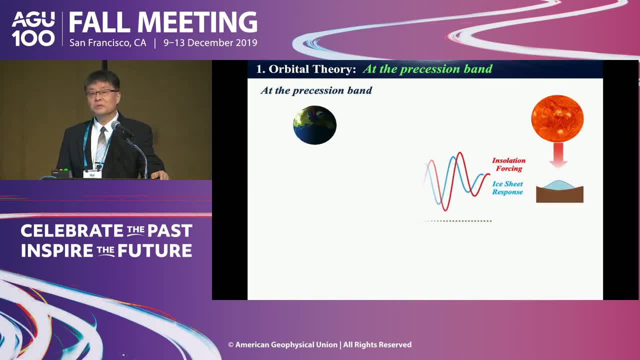 at precession band. At precession band that mean ice sheet response insulation forcing with 5,000 years lag. This lag is originally in Milakovic hypothesis as well as in Emiliani's data weighting record, But the lag has not been really well tested. 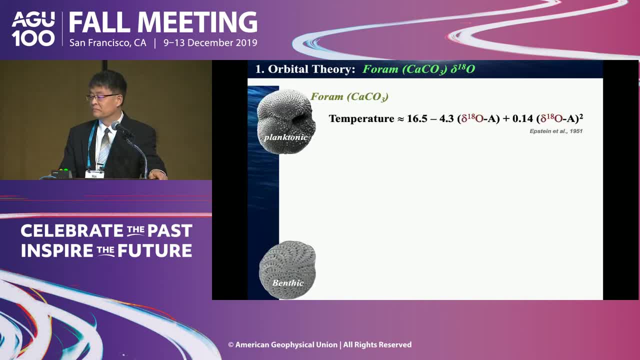 by absolutely dated climate proxy record. This is partially because the 4M, 4M itself, 4M can get temperature signal, no matter was the precision or accuracy it could. For example, this equation: this is the early version equation used by Emiliani: 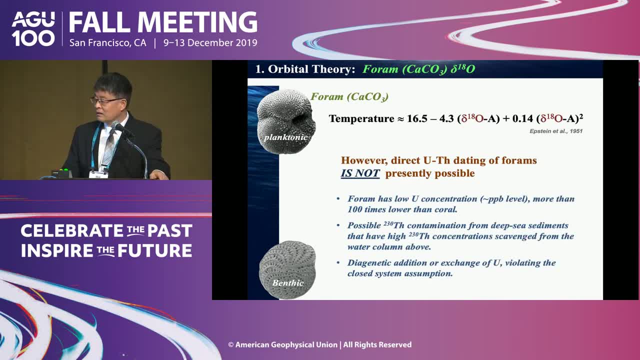 However, direct uranium and thorium dating of 4Ms is not presently possible because 4M has low uranium concentration, possible thorium-230 contamination and diagenic addition and exchange of uranium, which of course is sort of an open system behavior. 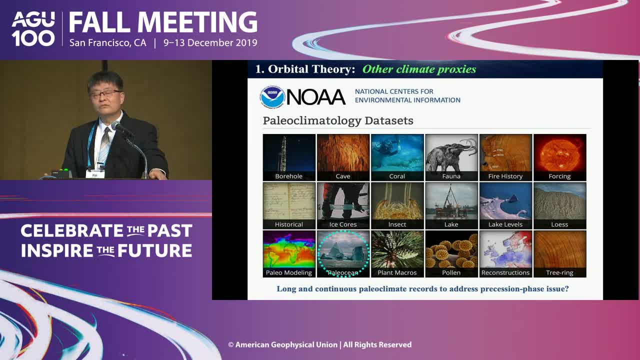 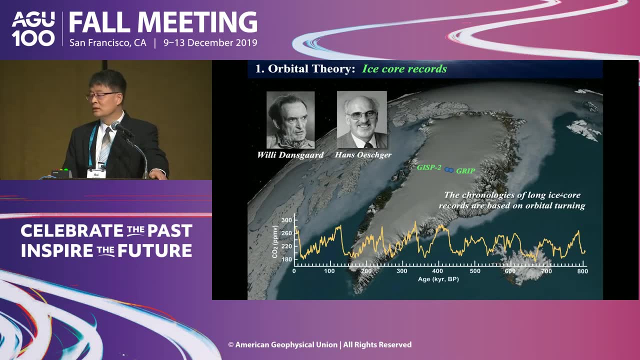 So, besides marine data weighting record, do we have long and a continual climate record to use? The answer is yes, of course. For example, ice core record is continuous and long enough now, but the chronology of long ice core record are based on. 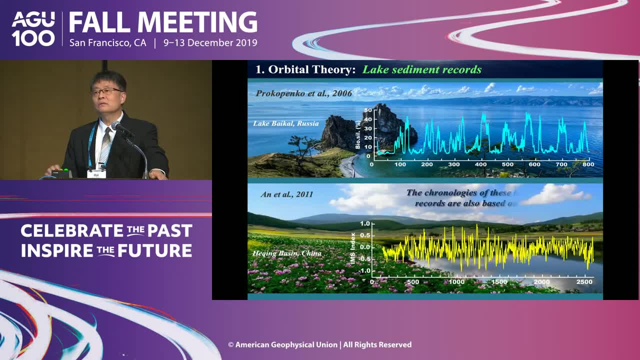 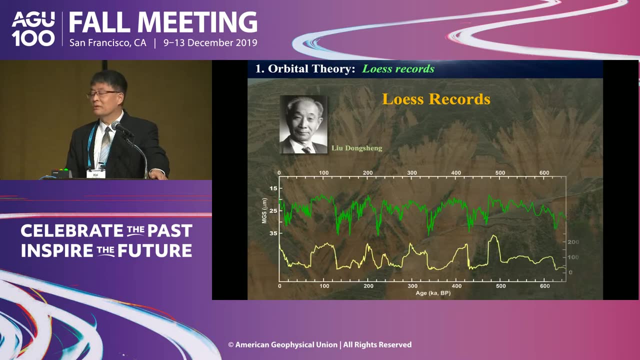 orbital turning. essentially, There are a bunch of long and a continual beautiful lake records. However, the chronology of this long lake sediment record are also based on orbital turning. This record is continuous and long enough, but chronology again based on the orbital turning. 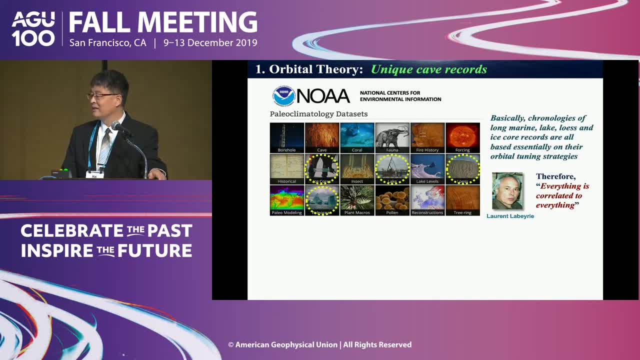 So, basically, chronologies of long marine lake, earth and ice core records are all based essentially on their orbital turning strategy. Therefore, everything is correlated to everything, which is good, probably the other side, which make it it difficult to resolve the phase difference. 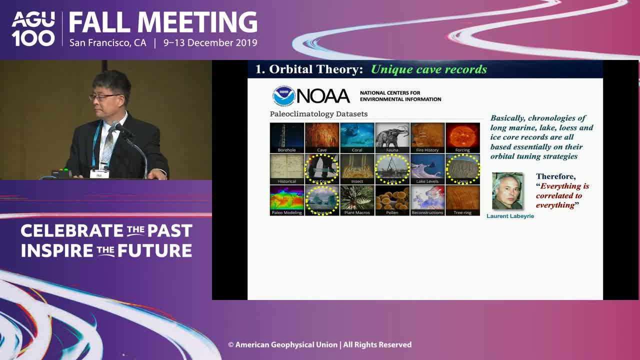 especially the precession phase differences. Therefore, do we really have a record with independent chronology or absolute dated chronology? The answer is also yes. Cave data weighting records are suitable for independent and absolute uranium and thorium, as well as uranium and lead recently. 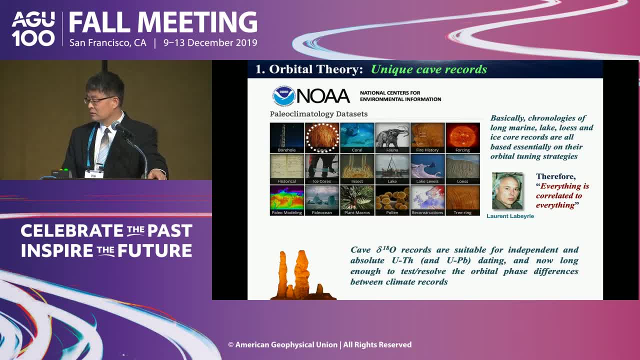 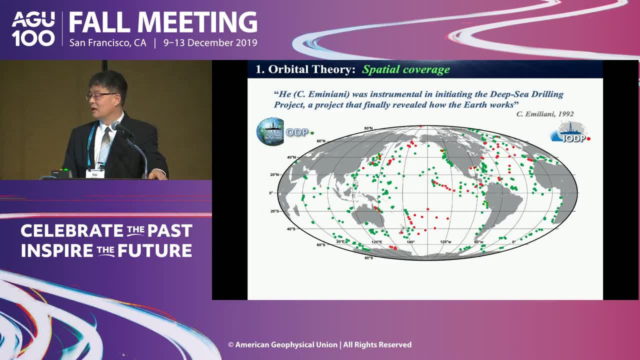 dating and now long enough to test the orbital phase difference between climate records. Regarding spatial coverage, Arminiani said a long time ago he himself was instrumental in initiating the deep sea drilling project, a project that finally revealed how the Earth works. 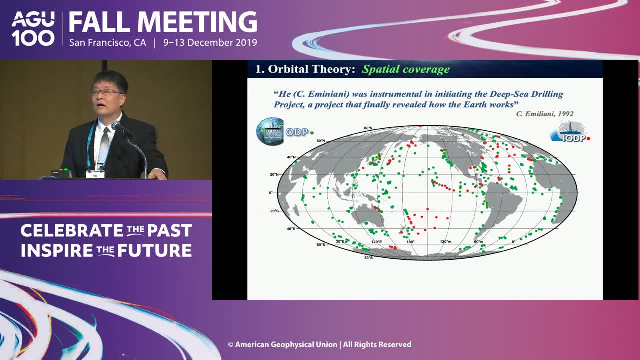 After that, then I think in the past. after that, then I think in the past. after that, then I think in the past. after that, the ODP and the IODP project indeed. 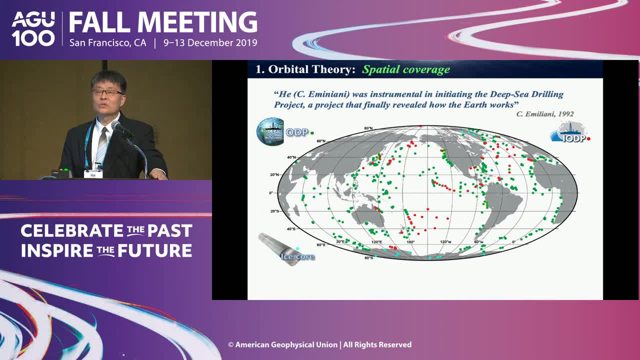 have covered the ocean globally, Then ice core record covered the north and the south polar regions, Greenland, Antarctica. In the past two 20 years cave data weighting record have covered most of land region become an important complement to marine and ice core record. 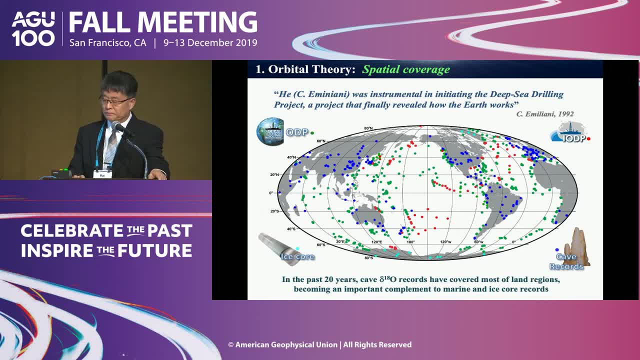 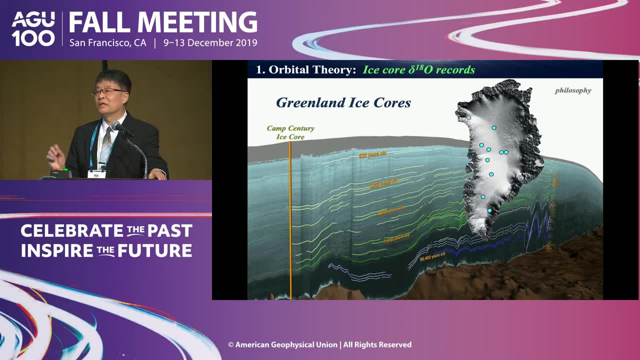 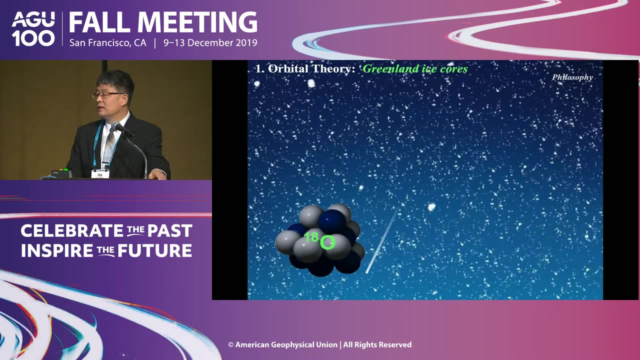 Therefore, now we do have a global view, People in our field familiar with ice core data weighting record, most of them. I mean paleo-ocean graphic or paleoclimate refuel, For example, Greenland ice core. This is probably because the snow has a lot of climate. 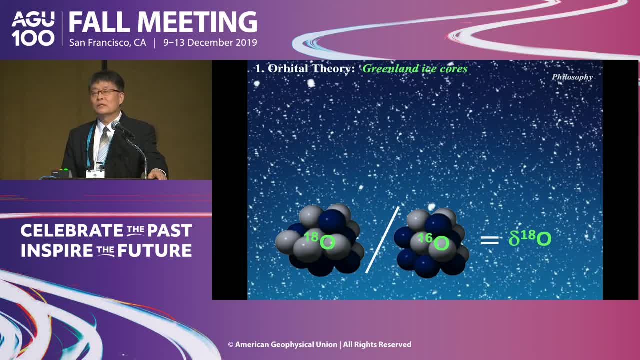 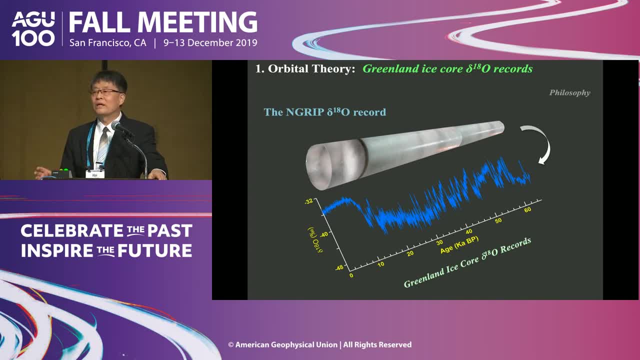 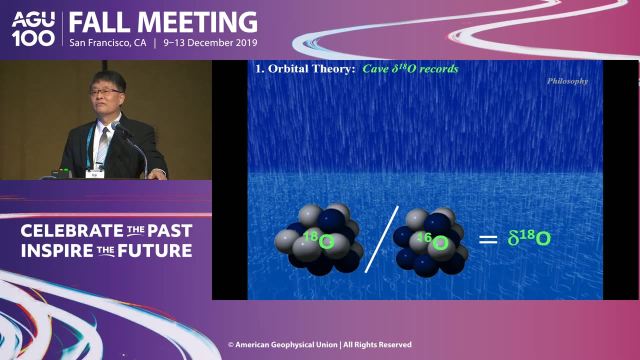 The snow accumulates in the polar region turns to ice gradually. you drill an ice core and measure the ice delta weighting. you get an ice core delta weighting record. For example, this is N-gripper record In low and the middle latitude. however, we do not have snow accumulation. However, we do have a lot of rainfall. Rainfall has similar climate signals, such as delta weighting. Most of the rainfall evaporate back to air or run off back to ocean. However, there are tiny portion of those rainfall water. 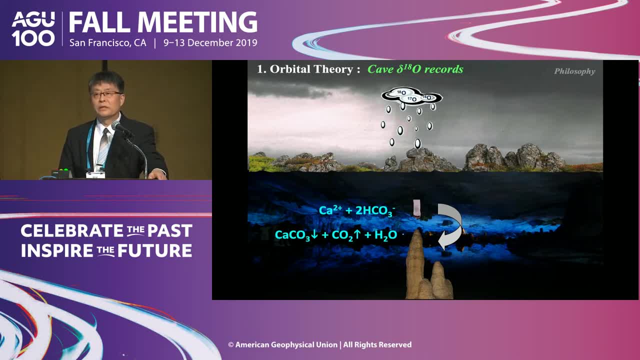 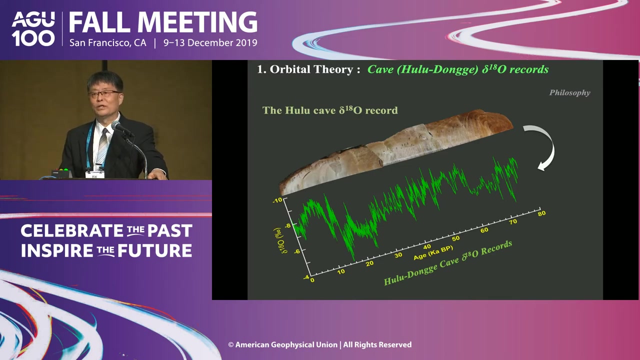 get into cave system involving the formation of a symbolism. Essentially, this process propagate delta weighting of rainfall to the groundwater or dripping water and eventually fix this delta weighting signal into the symbolism. If you get a sample of symbolism and cut it and polish it and measure carbonate, this delta weighting. 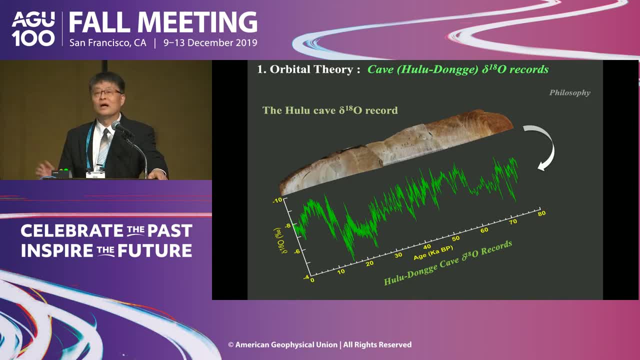 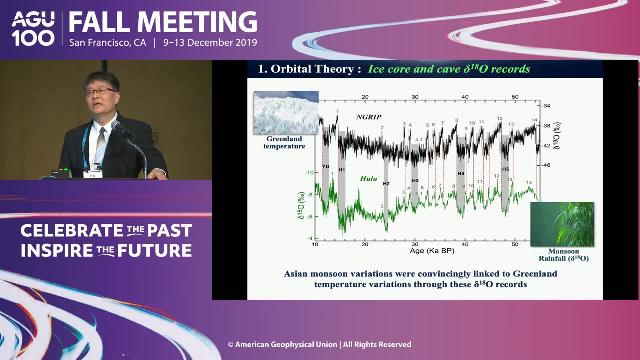 you get a cave delta weighting record, such as a Hulu record. as I mentioned before, Both ice core delta weighting record and cave delta weighting record are equally important. For example, you use both records, you could get the Asian monsoon variation. 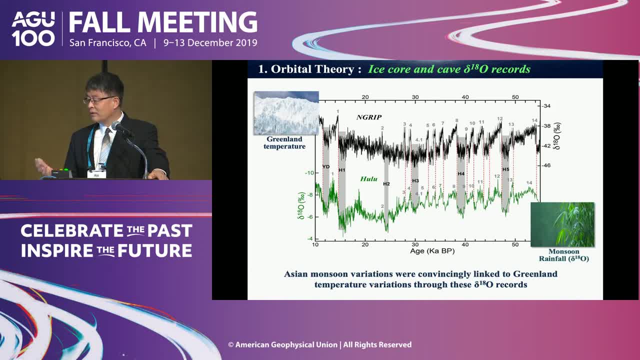 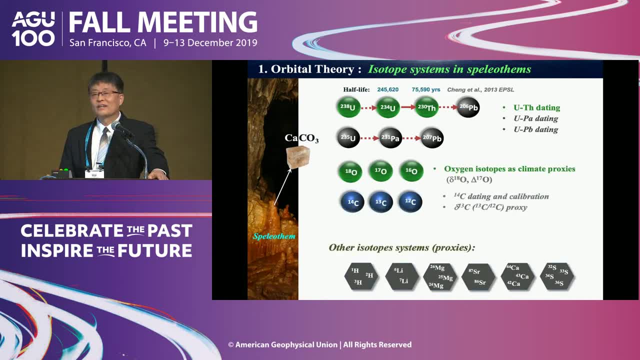 And the Greenland temperature record and correlate them convincingly together. Spillism in general is calcite or arachnid. These minerals contain a lot of isotope system that is very useful for paleoclimatic research. However, here I only can mention uranium-238 decay chain. 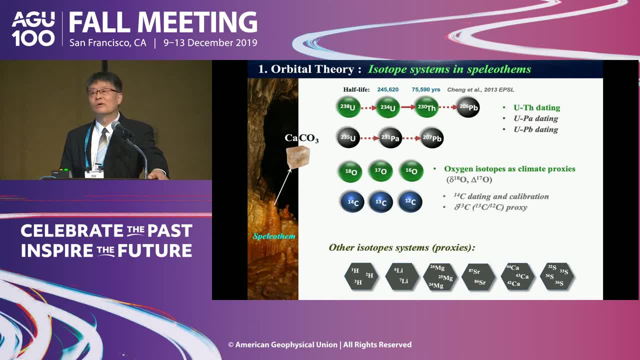 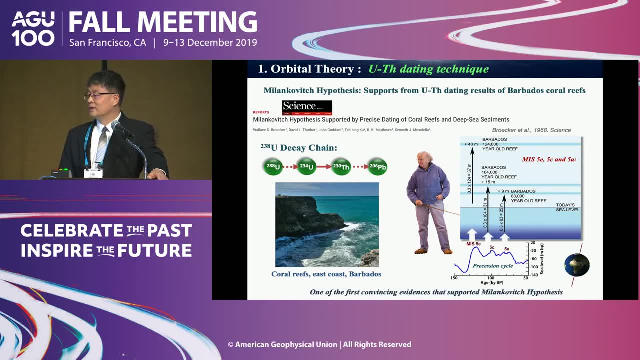 for uranium-saurium dating And the oxygen isotope for the climate proxy In the early stages. uranium-saurium dating is always powerful. For example, Wally and his colleague dated the coral reef in 1968, and they immediately found precession cycle. 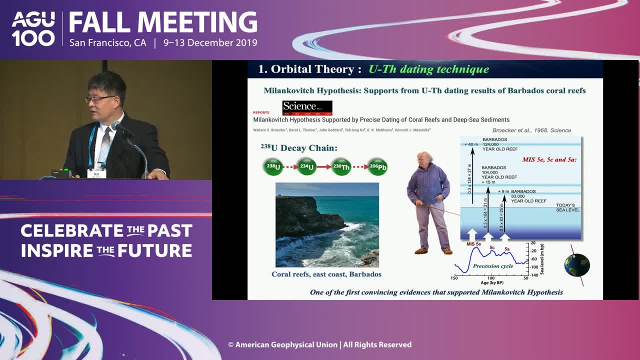 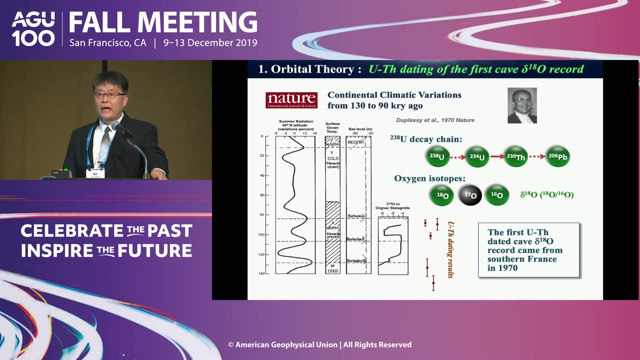 of a sea level change like 5E, 5C, 5A, provided one of the convincing evidence that supported the Milakovich hypothesis. Okay, in our field, this first uranium-saurium dated cave delta weighting, I believe. 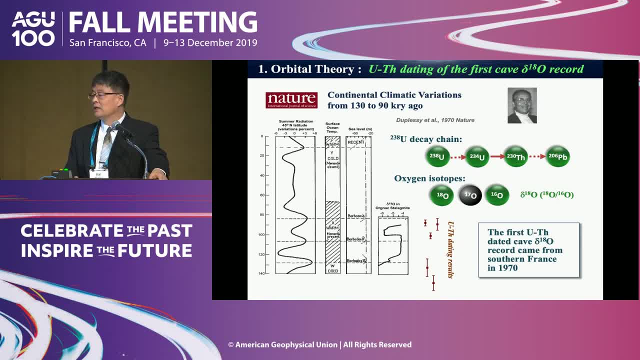 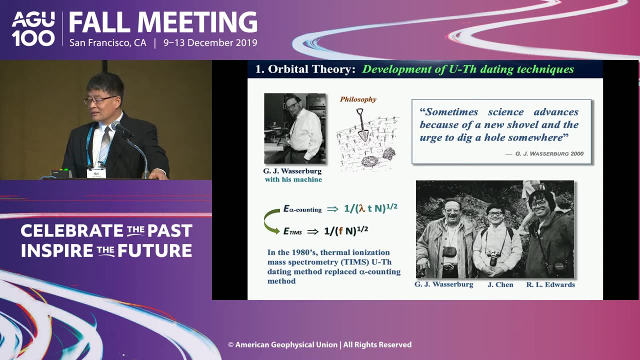 came from southern France in 1970, which characterized continental climate variations from 130 to about 90,000 years ago. In 1980s, the uranium-saurium dating method replaced the early alpha counting method and the Washenberg, Chen and Larry Ellis. 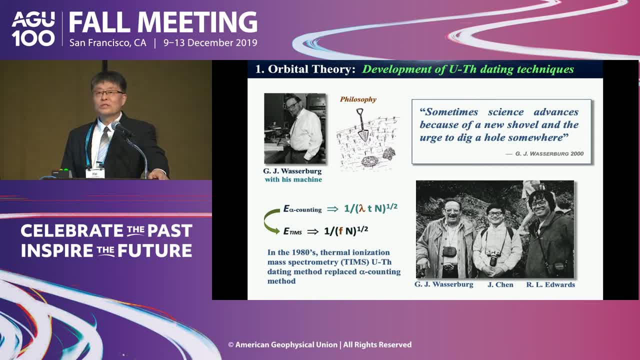 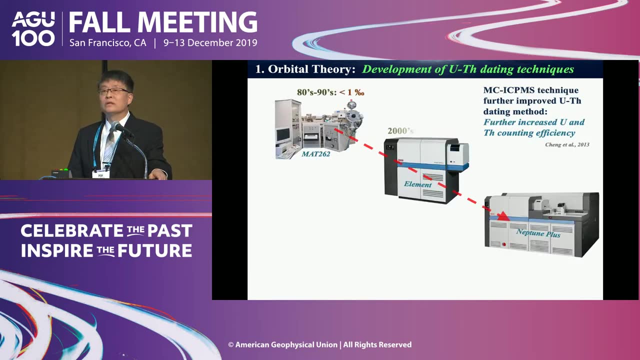 did substantial contributions. Later, Washenberg commanded this development. to say that sometimes science advances because of a new shovel, this method, basically, and the urge to dig a hole somewhere Recently. multi-collector ICPMs. multi-collector ICPMs. 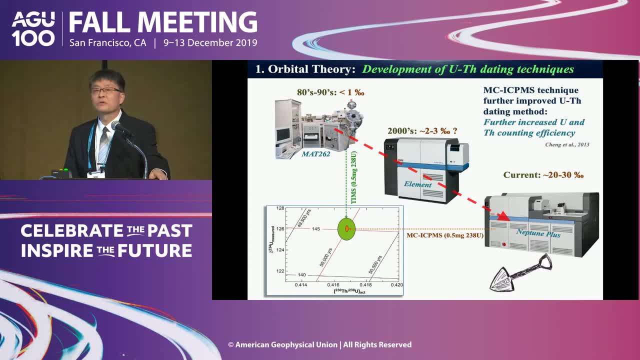 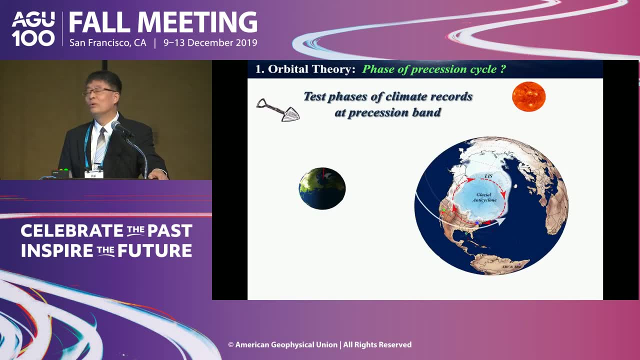 this technique further improved the uranium-saurium dating. Now we do have a new tool and the urge to dig a hole somewhere. What we could do first thing, I thought, is test the phases of climate records at precessions band. 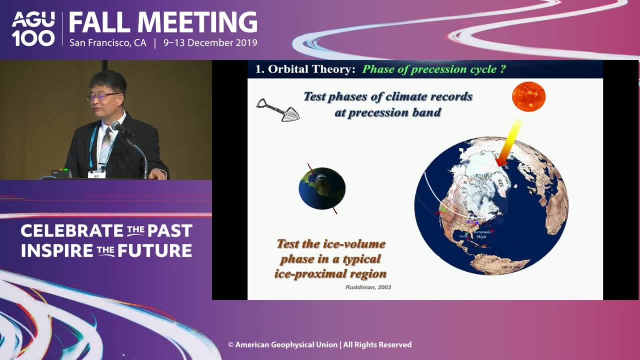 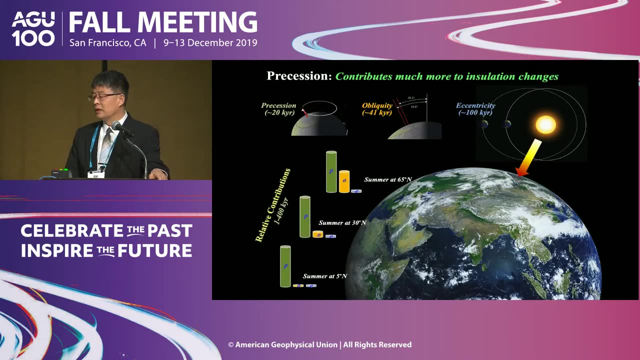 For example, to test the ice volume phase at a typical ice proximal region such as in this country, West Virginia. why precession? Precession actually contribute much more to insulation changes from low latitude to middle latitude, even to high latitude. 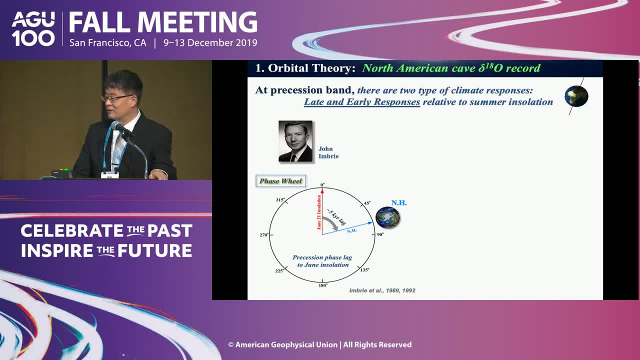 At precession band. there are two types of climate response. we called later and early response relative to some insulation. This is a phase wheel to show precession phase lag to June or summer insulation According to Inbrail. Northern Hemisphere climate change. 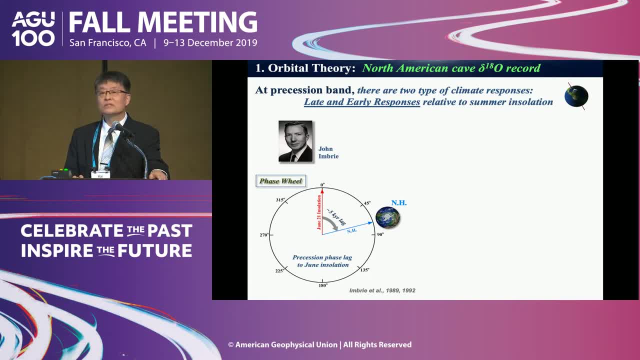 lags summer insulation by about 5,000 years. They also noted there are some climate change of like shorter or shorter, like early response, like Southern Hemisphere SST. Later Rudiman emphasized that in ice-proximate regions climate change lags to June or summer insulation. 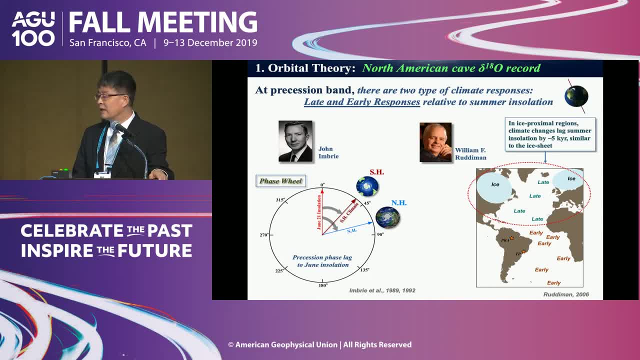 So lags summer insulation by 5,000 years, similar to ice sheet. Therefore, we think this cave record gonna be very important, because we call it the BCC- okay, West from West Virginia- because it simply close, very close to the ice sheet. 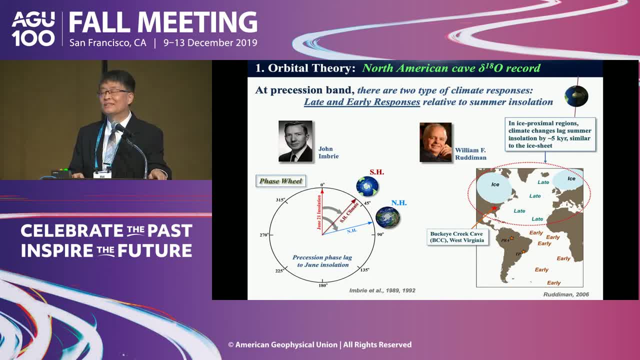 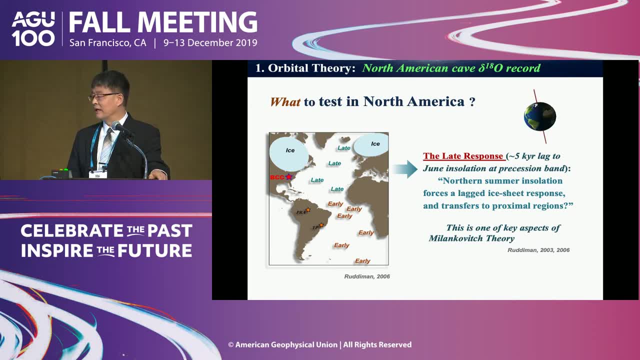 but not underneath the ice sheet, Otherwise you won't have spittism growth, okay. So what's the test in North America? First, of course, the late response: 5,000 years lag to summer insulation, Or northern summer insulation forces a lagged ice sheet. 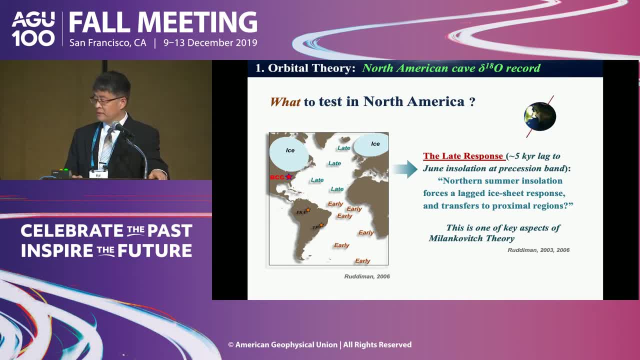 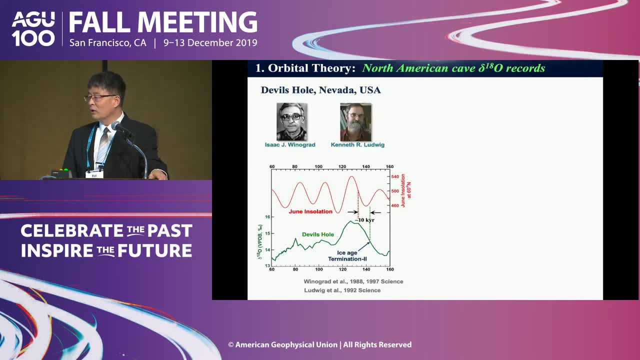 response and the transfer to proximal regions. This is one of the key aspect of actually the Malkovich theory of climate. Okay, in North American cave record there is a very famous early stage work from Davis Hall And it show that termination- ice age termination too. 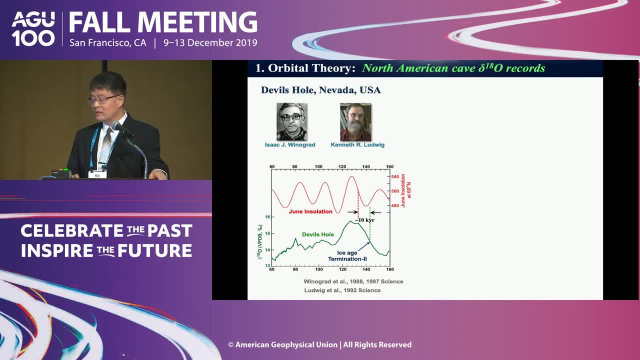 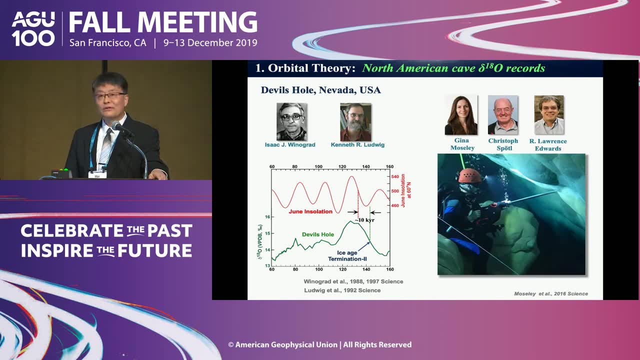 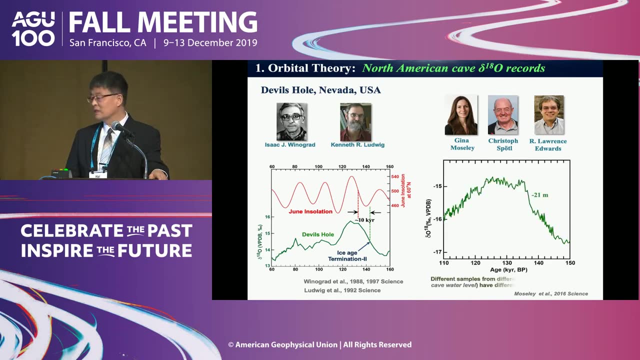 sort of lead insulation rise by 10,000 years, which challenge Malkovich theory. Recently, another group- okay- went back to the same cave and get a bunch of new samples. What they found is that different samples from different depths have different timing. 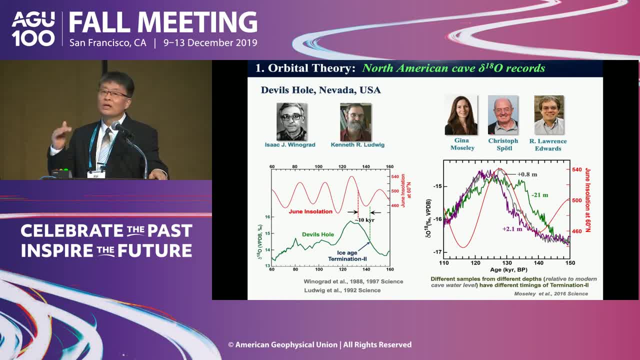 of termination too. They believe the shallow sample, like a 2.1 meter above the current cave level, is most reliable. okay, Therefore it lagged insulation, but the insulation in terms of precession phase is still clear. 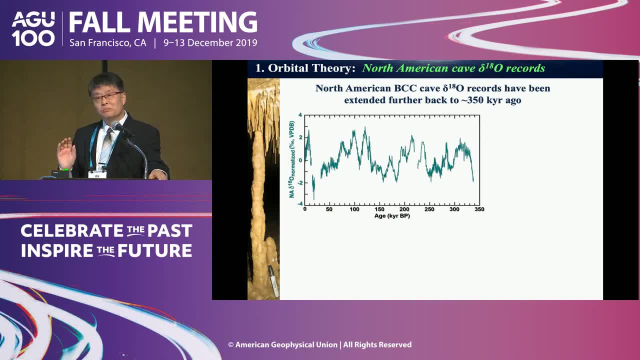 In this year we established or we pushed the BCC cave further back into like 150,000 years. Therefore we have longer enough record to test the phase of a precession band. What we found is that at precession band 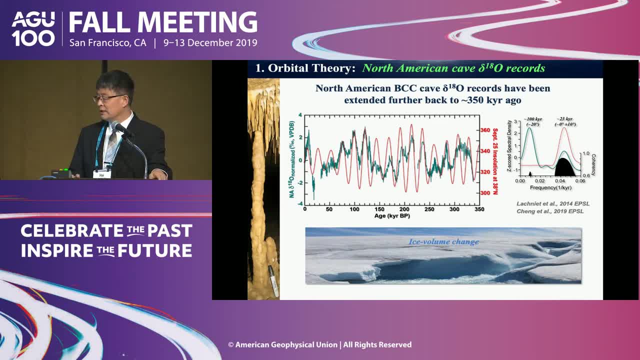 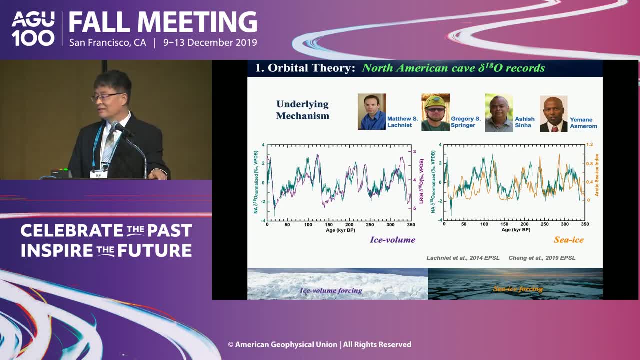 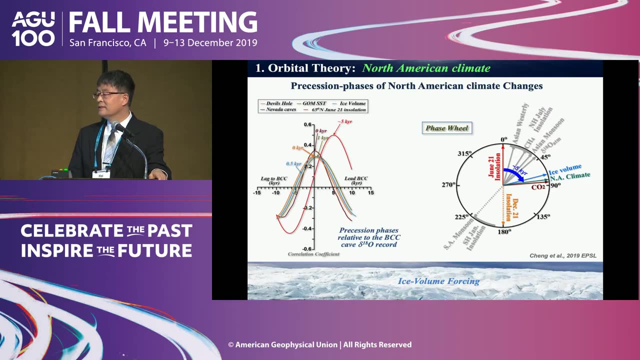 the in phase with sub-tempo insulation, therefore consistent with ice volume change, Underlying mechanism was considered as the like ice volume forcing and together with sea ice forcing. This diagram, the left one, show the precession phase relative to BCC. 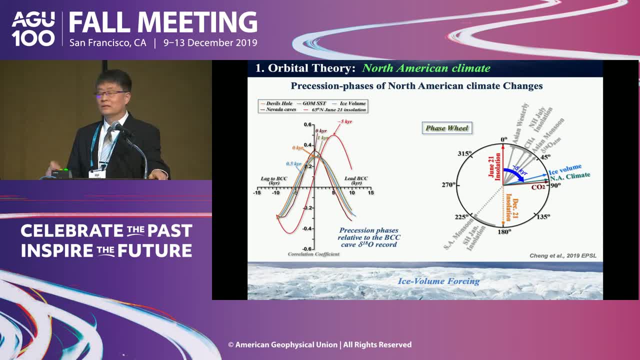 the cave delta weighting record and the precession scale. So you can see that precession phase of North American climate change, including Davis Hall, the new data and Gulf of Mexico SST ice volume, Nevada Caves seems to have same phase. 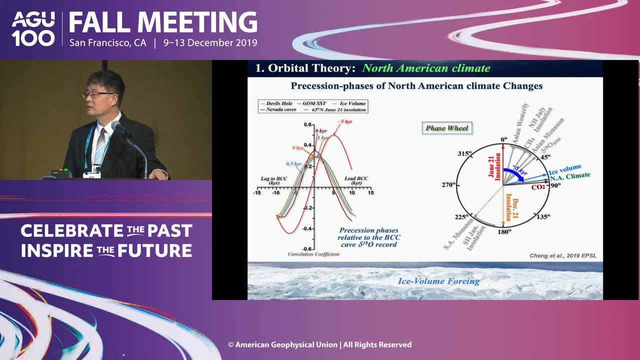 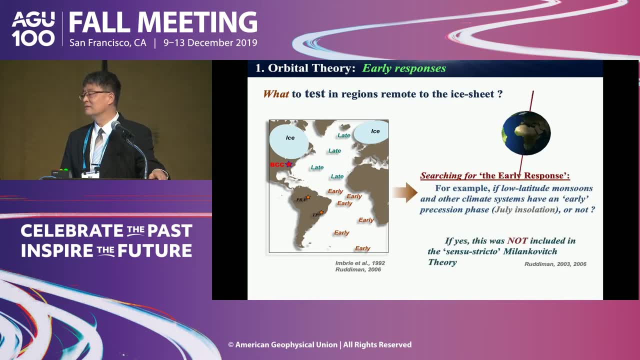 relationship with 5,000 years lag to the summer insulation. Then what to test the region remote to the ice sheet? We want to search for the early response, for example, the low latitude, monsoon variation and other climate variation at precession band. If yes, I think this was not including in the sense of stricto Milakovic's theory. So in monsoon regime, a classical wisdom from John Kurzbach is this: the monsoon rainfall are in phase with the summer, of July insulation. 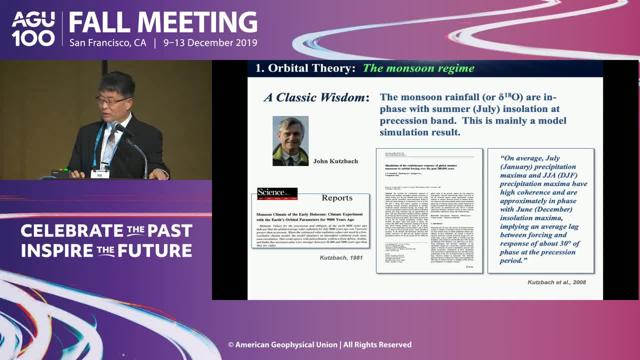 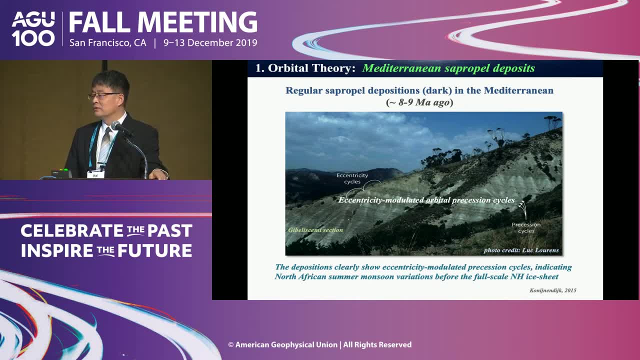 at precession band. This is mainly from the model simulation result And the in real world you also can see this scenario directly. For example, the regular sepropyl deposits in the Mediterranean, like eight to nine million years ago, demonstrated that the 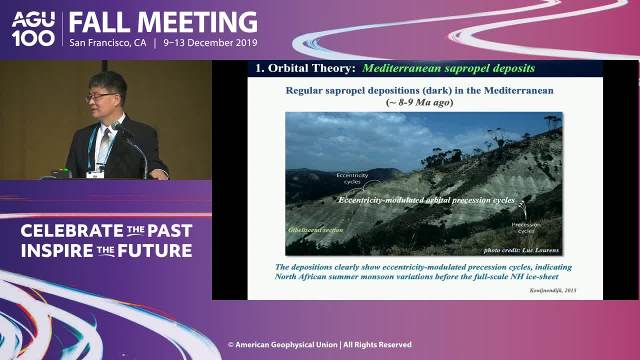 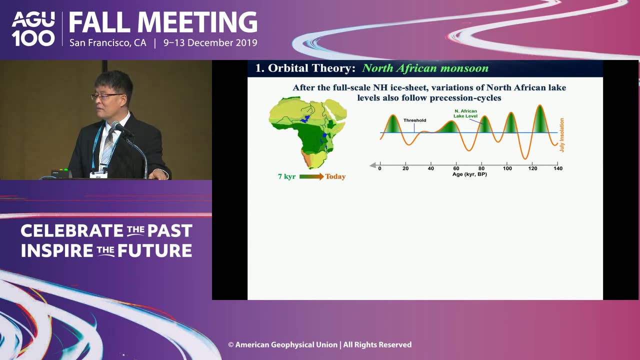 eccentricity modulated orbital precession cycle clearly, which indicates northern Africa summer monsoon variation. before the full scale northern hemisphere ice sheet. After the full scale northern hemisphere ice sheet. variations of the North Africa lake levels also follow precession cycles. 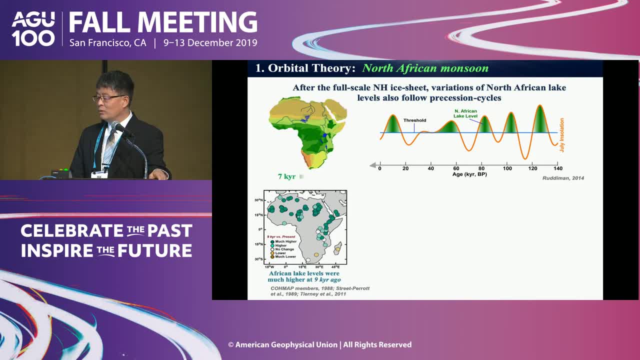 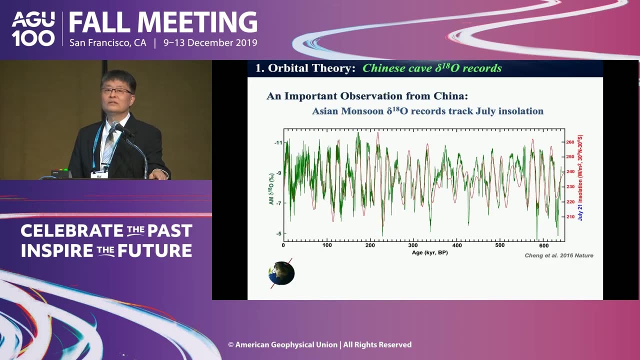 For example, African lake level were much higher at 9,000 years ago And the sepropyl record also showed that the Northern Africa summer monsoon follow some insulation In China. an important observation recently is that the Asian monsoon data weighting tracks the July insulation. 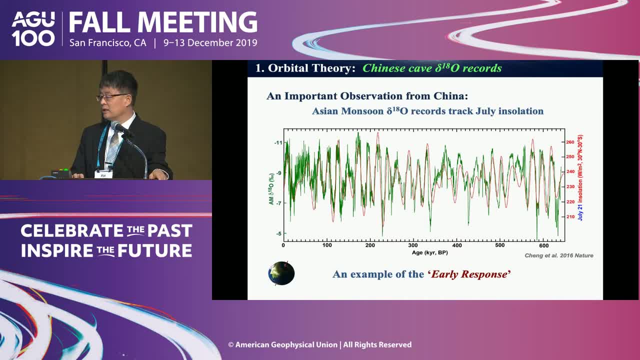 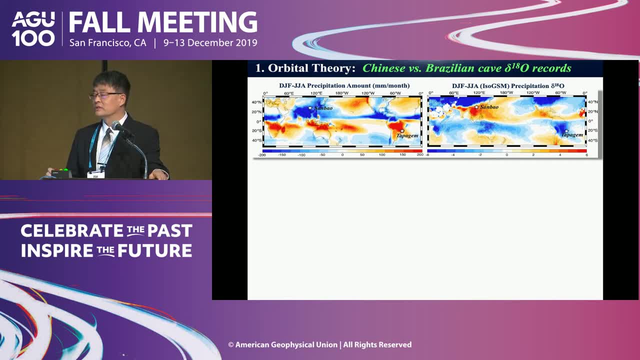 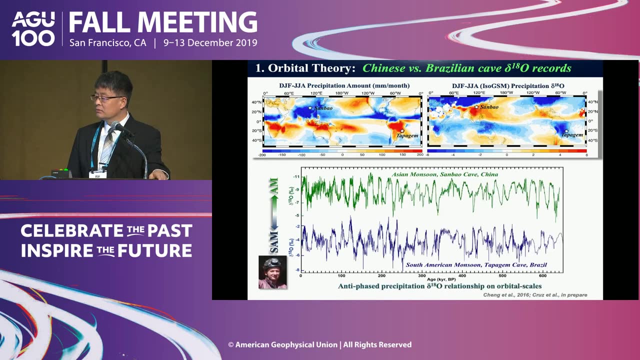 which provide a robust early response. example: Okay, this diagram shows the inter hemisphere contrasting of the seasonal precipitation amount and the seasonal precipitation data weighting: The record from the Sanbao cave. the top green curve is from China, northern hemisphere. The bottom curve is the Tapachi cave record. 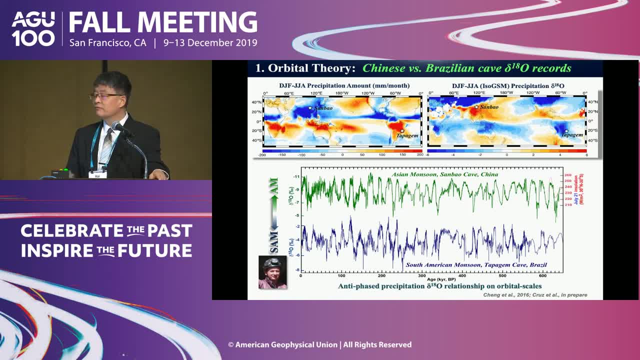 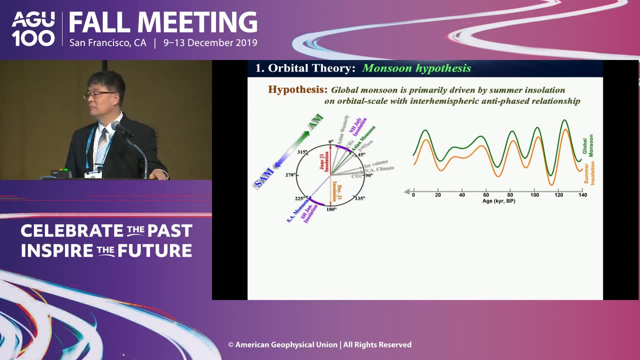 from Brazil in southern hemisphere. They follow northern hemisphere insulation and the southern hemisphere insulations respectively. therefore display antiphased precipitation data weighting relationship on orbital scale. Overall, we do have monsoon hypothesis that global monsoon is primarily driven by summer insulation on orbital scale. 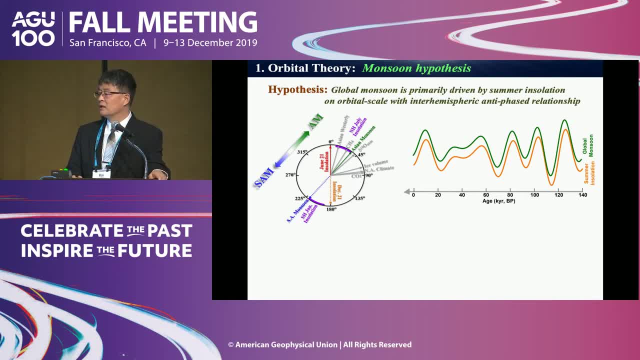 with inter hemisphere antiphased relationship. This is the simplest hypothesis, which I think tends to be right If you believe Occam's razor, which is, all things being equal, the simplest solution tends to be the best one. In addition, we also found that the Asian westerly climate 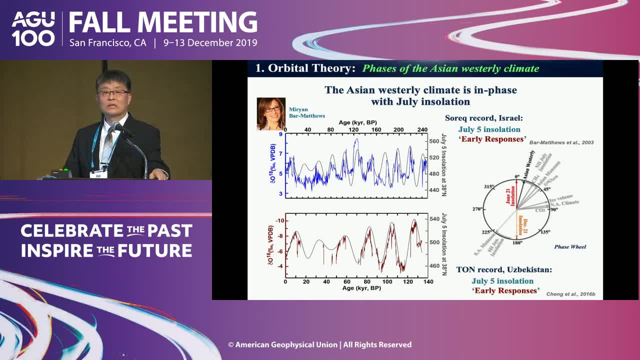 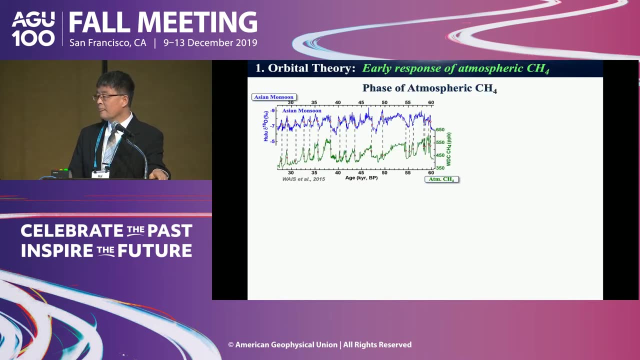 is also in phase with July insulation. For example, the cave record from a Sarek cave, Israel, or cave record from a town record in Uzbekistan. Central Asia. We knew that Asian monsoon data weighting record has greater or very close than the Asian monsoon data weighting record. 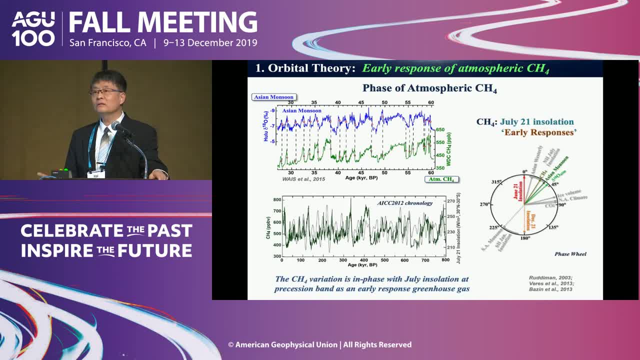 This is a close relationship with the atmospheric method On longer time scale or orbital scale. we also can confirm that the method variation is in phase with the July insulation at precession band as an early response greenhouse gas. They are very close to Asian monsoon. 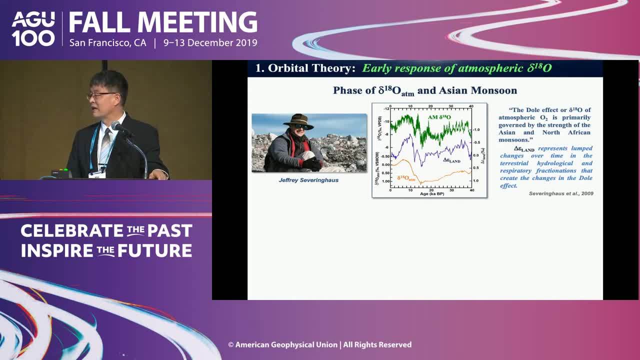 10 years ago, Jeff Savinghouse found that the Doa effect- or data weighting of O2, is primarily controlled or governed by the strength of the Asian and the North African monsoon On the long time scale or orbital scale. we also confirm that data weighting of atmospheric O2 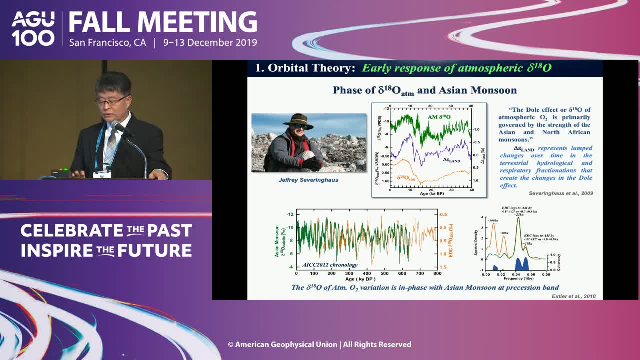 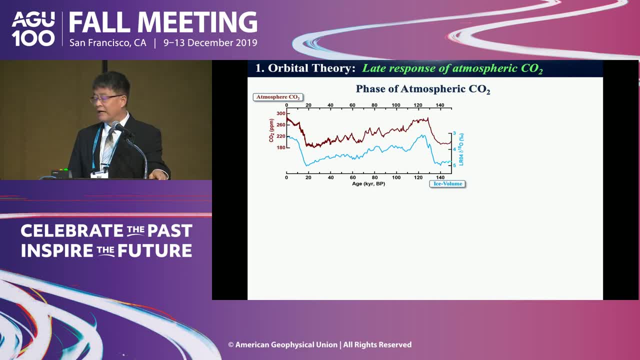 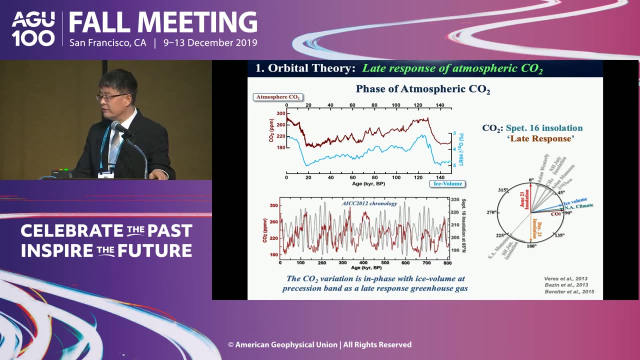 variation is in phase with Asian monsoon at precession band. We also knew that atmospheric CO2 has close relationship with ice volume. so we also found on the orbital scale CO2 variation is in phase with ice volume at the precession band. as a later response, greenhouse gas. 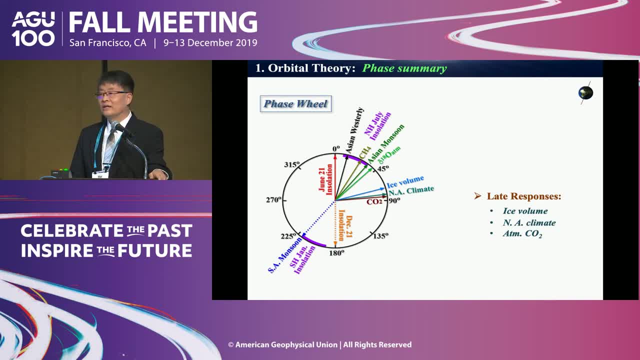 The overall. we see later response as predicted, like ice volume, like North African American climate and atmospheric CO2.. We also see a bunch of early response like monsoons, southern hemisphere, SST- I'm not quite sure okay. 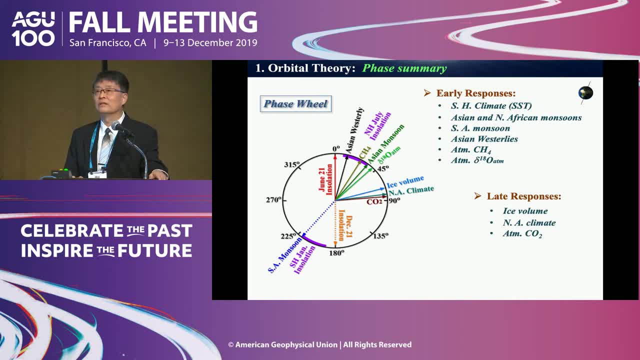 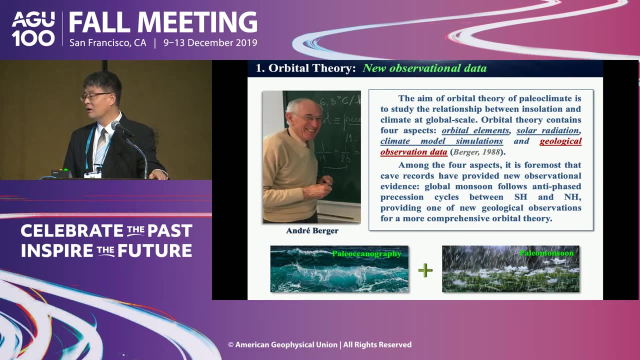 But we see the variation of the atmospheric methane and the data weighting of CO2.. So the question here is really this: the early response are not really included in Milakovic's theory of climate yet. So, according to Andrew Berg, the aim of the orbital theory of paleoclimate 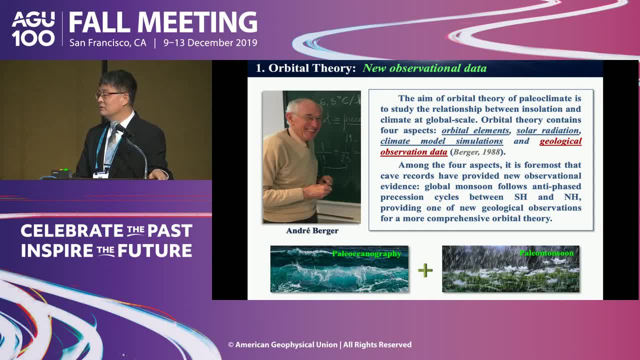 is to study the relationship between insulation and the climate at a global scale. The orbital theory contains four aspects: Orbital elements, of course, solar radiation, climate model simulations and geological observation data. Among the four aspects, it is foremost that the cave records have provided. 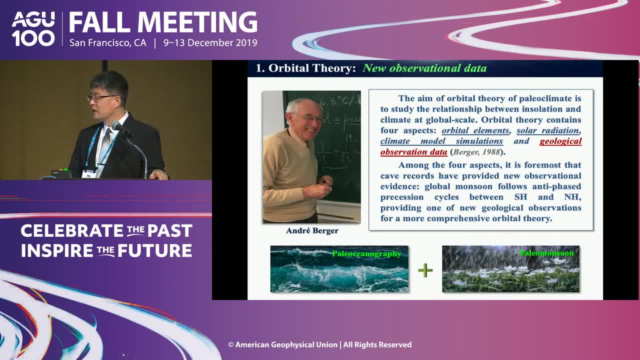 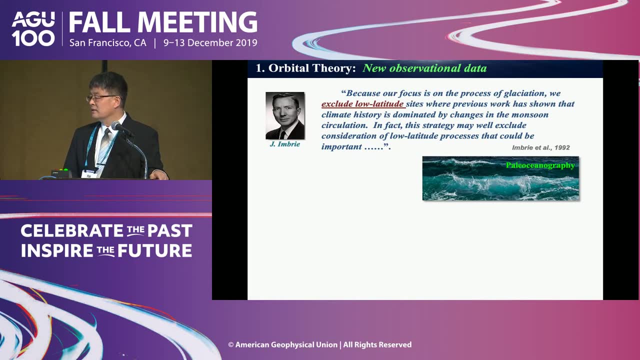 new observational evidence: global monsoon deaths Follows anti-phase precession cycles between south and the north hemisphere, providing one of the new geological data- geological observations- for a more comprehensive orbital theory of climate. In 1992, Inbre wrote. 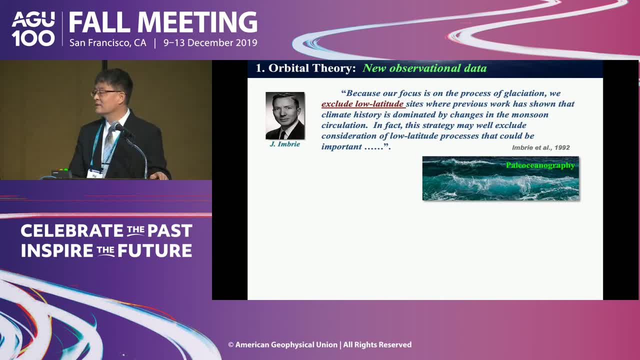 because our focus is on the process of a glaciation, we excluded low latitude site, where previous work has shown that climate history is dominated by change in the monsoon circulation. In fact, this strategy may well exclude the consideration of a low latitude site. 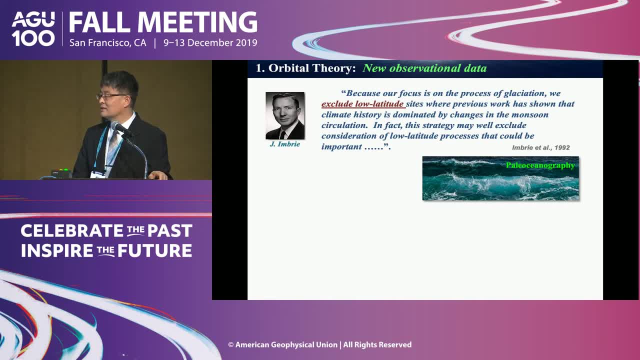 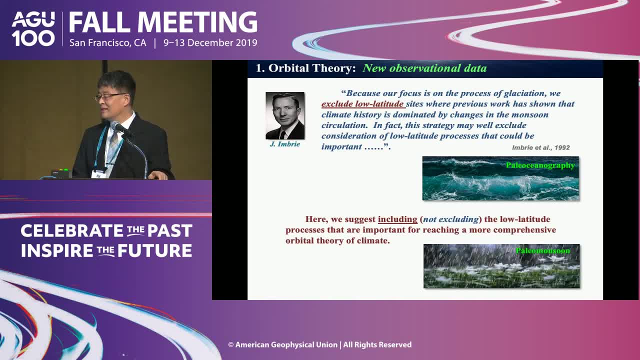 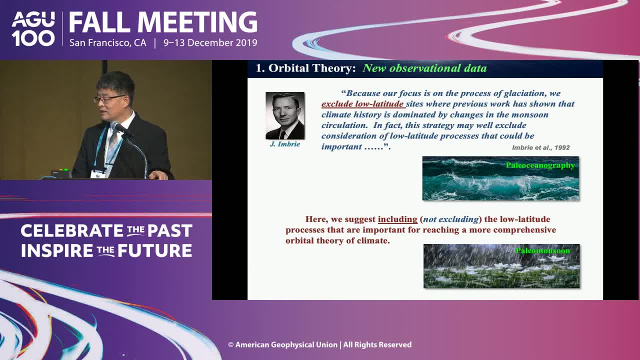 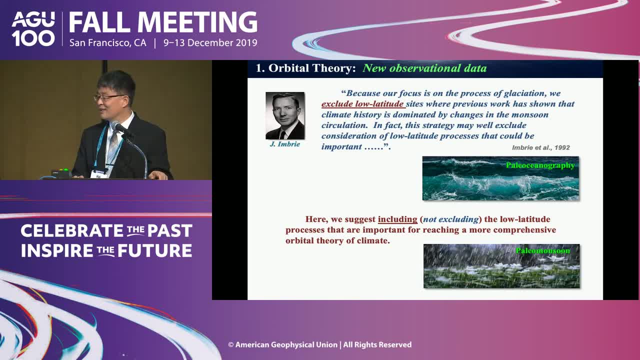 In fact, this strategy may well exclude the consideration of a low latitude site. In fact, this strategy may well exclude the consideration of a low latitude site. to me, for reaching a more comprehensive orbital theory of climate, Here is a list of milestones in evolution. 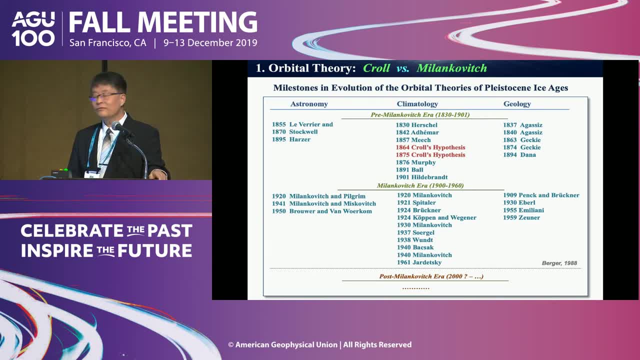 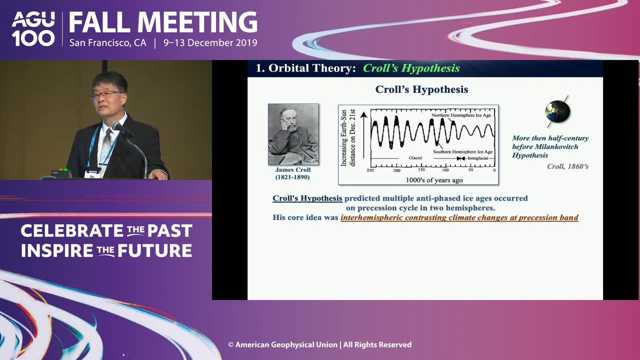 of the orbital theories Of note is cross-hypothesis. Cross-hypothesis is important because it predict multiple antiphase. ice age occurred on precession cycle in two hemisphere. His core idea was inter-hemisphere contrasting climate changes at the precession bend. 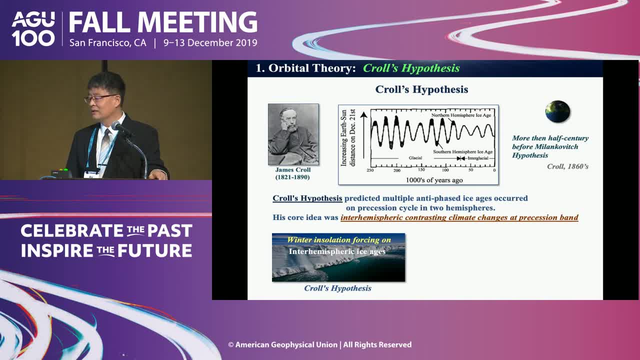 He emphasized the winter insulation forcing on inter-hemisphere ice age, which was wrong. But recently K record also showed the core idea: like summer insulation forces summer, not winter- on inter-hemisphere monsoons, not ice ages. 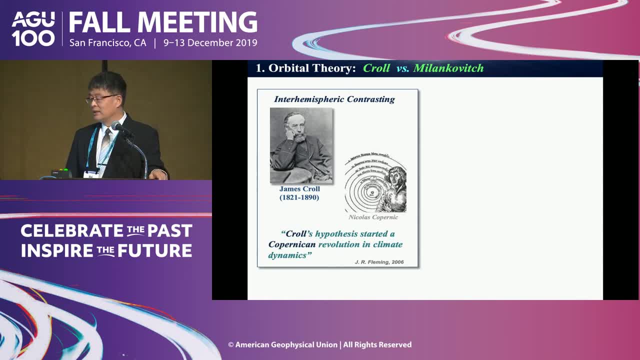 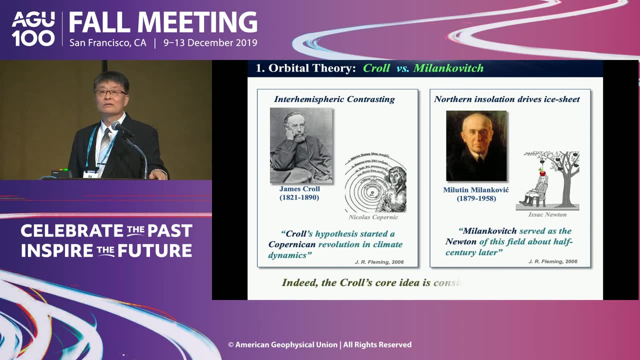 So that's probably why 2006,, to get Jim Flaming commented that cross-hypothesis started Copernican revolution in climate dynamics, and while this, Milakovic served as the Newton of this field, our field, about a half century later. 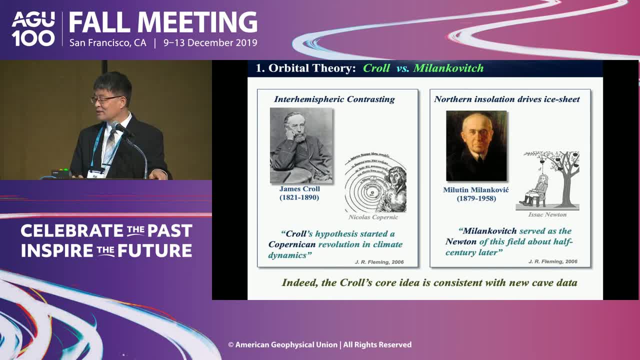 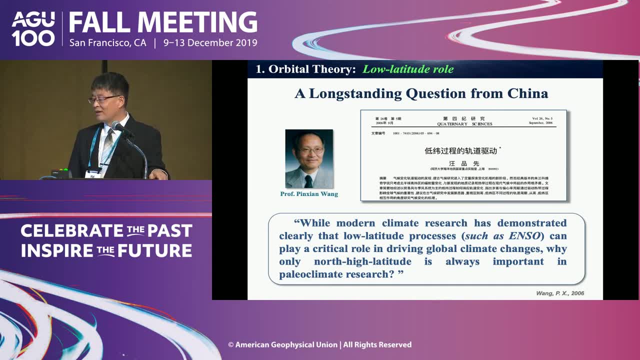 Okay, indeed, the cross-core idea is consistent with the K new K data In China. there's a long-standing question, that is, while modern climate research has demonstrated clearly that the low latitude process, such as ANSO, can play a critical role in driving global climate change. 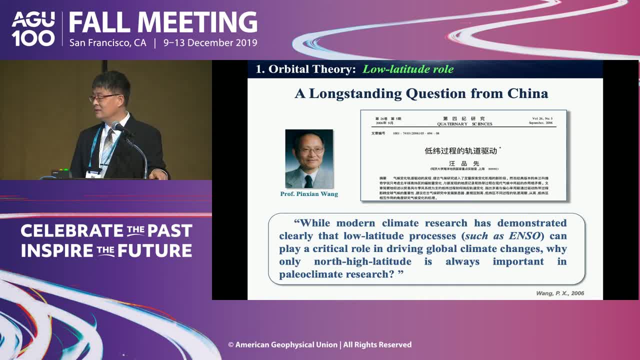 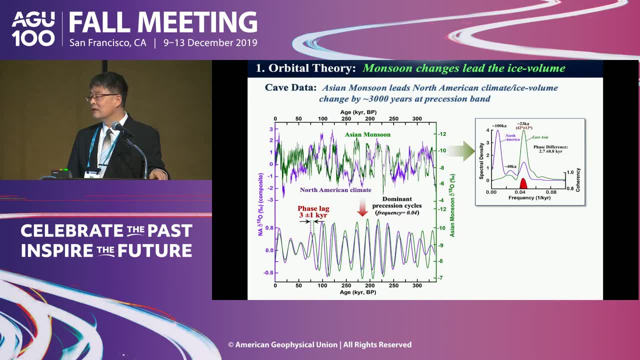 why only not? high latitude is obviously important in paleoclimate research. Okay here new K data show Asian monsoon leaves ice volume change by 3,000 years at precession. bend Those two records from North African, no American. 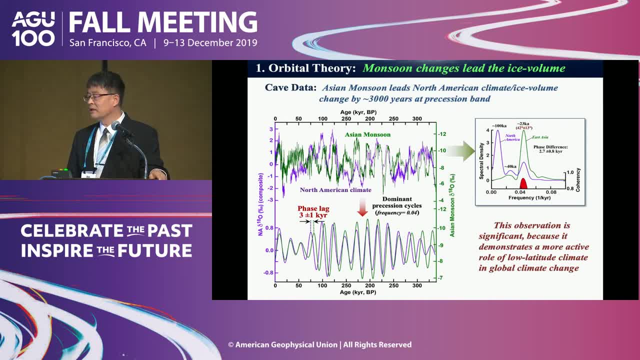 and Asian monsoon. the dominant precession cycles really have like 3,000 years plus minus 1,000 years differences with Asian monsoon. leave the North American Climate. This observation is significant because it demonstrate a more active role of low latitude climate. 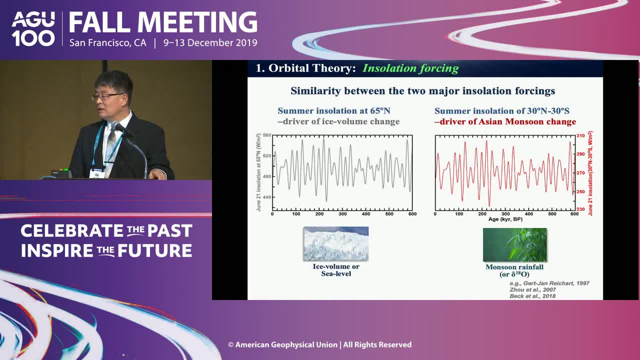 in global climate change. Regarding insulation forcing, there is very important or interesting similarity between the two major insulation forcing. One is the summer insulation at a 65 degree north, which is considered as a driver of ice volume change. Okay, That is the summer insulation of the 30 degree north minus. 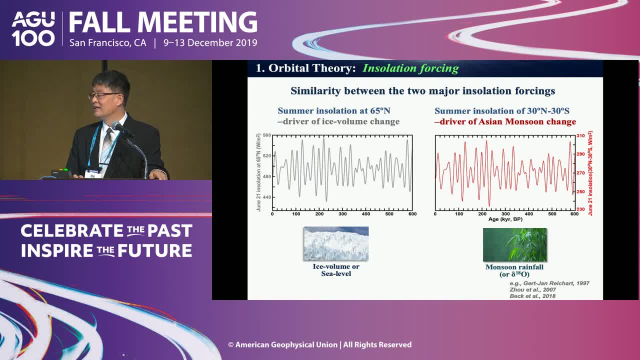 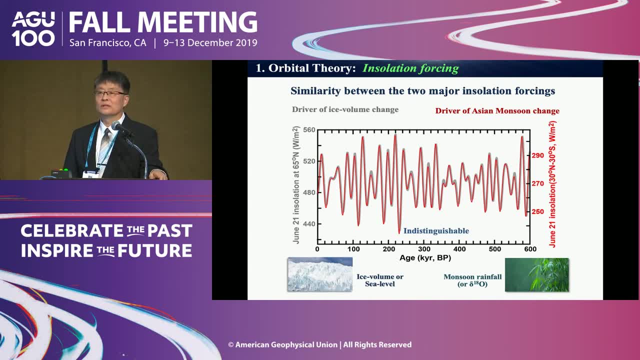 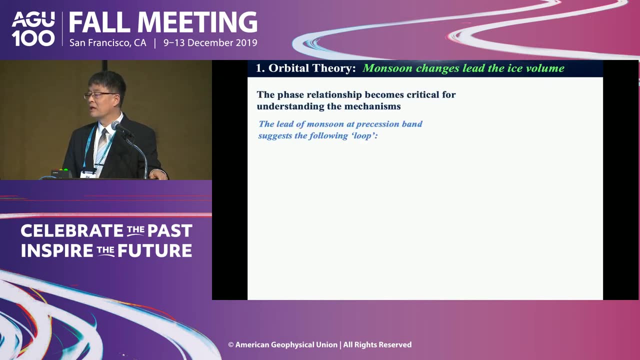 30 degree south considered as a monsoon driver. Okay, however, those two forces virtually indistinguishable, They are just overlapped. So therefore, the phase relationship became so critical for understanding the mechanisms The leader of monsoon at precession bend suggested. 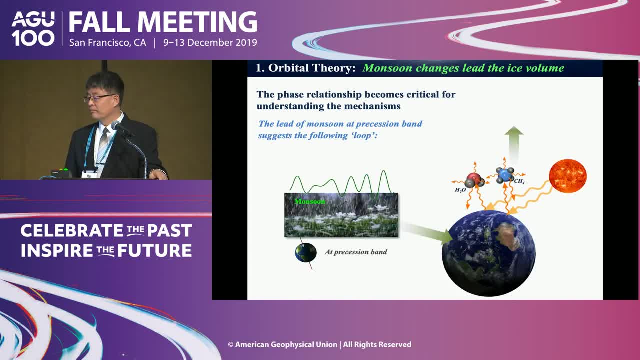 the following loop: At precession bend, the monsoon intensification might cause the rising of water vapor in atmosphere, which may act as a additional force to ice sheet decay. Ice sheet decay might act as a positive feedback through CO2 and the temperature to further intensify the monsoon variation. 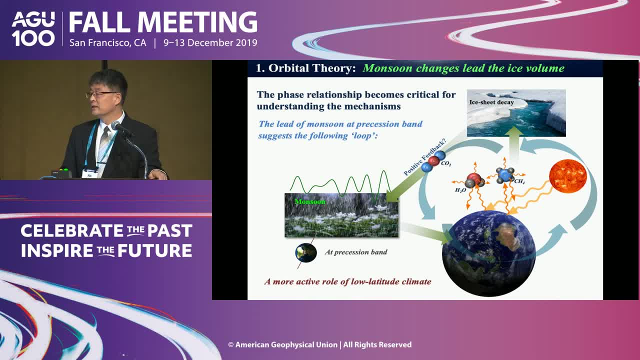 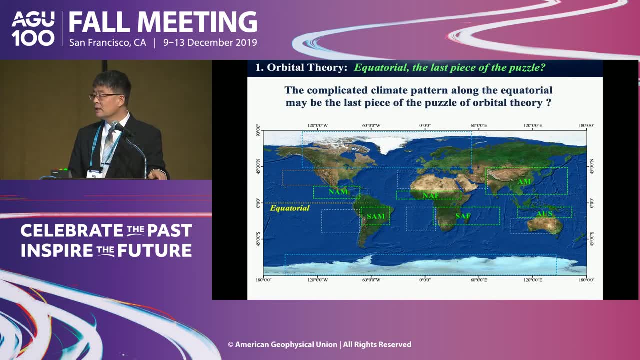 Anyway, the loop is this directionality, not the opposite, Therefore suggesting a more active role of low latitude climate. I want to mention one thing, that's around the equatorial. The complicated pattern may be the last piece of the puzzle of the orbital system. 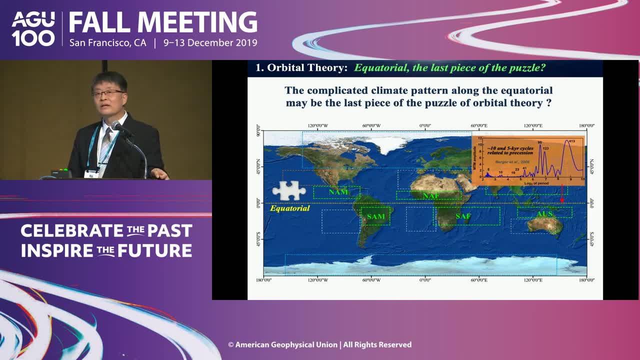 The first piece of the theory for me. I didn't see very clear evidence for 10 and 5,000 years cycle, as predicted, And instead we see some South American dipole on precession scale, but only in interglacial, not in a glacial time. 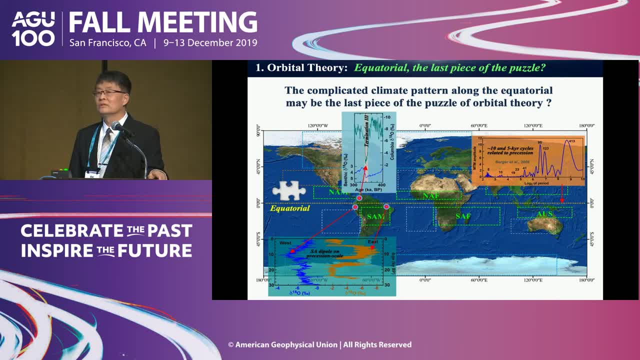 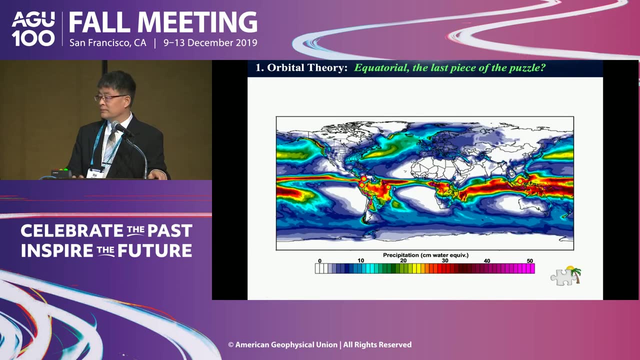 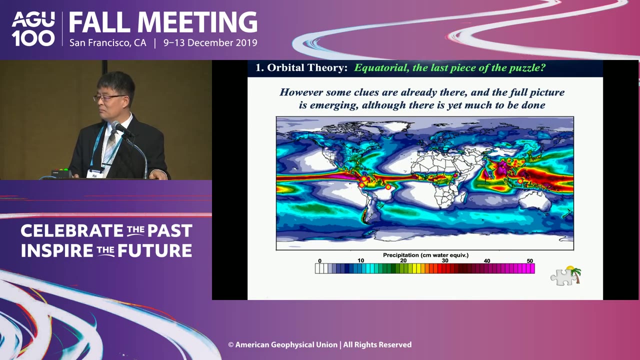 We also see some very large excursion of termination from Columbia- eight per mil or even large- And we see some kind of unusual long MIC-11 from Borneo at central. However, some clues are already there, I believe, And the full picture is emerging. 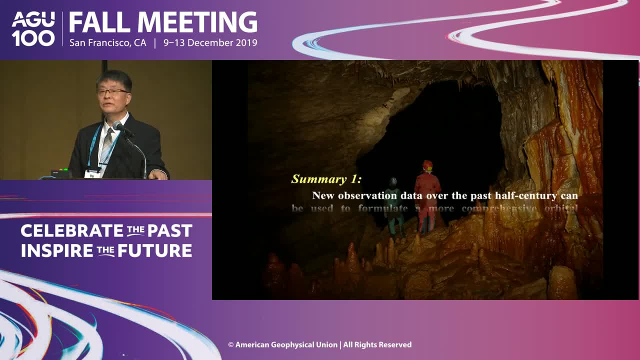 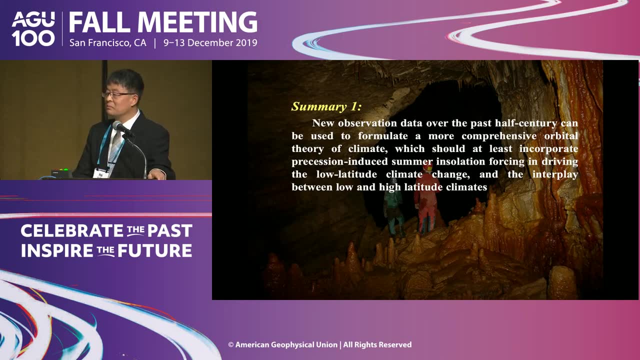 although there is yet much to be done, Here is my first summary: new observation data over the past half century, And I think it's important to note that this is the first time I've seen this kind of observation data And I think it's important to note that this kind of observation. 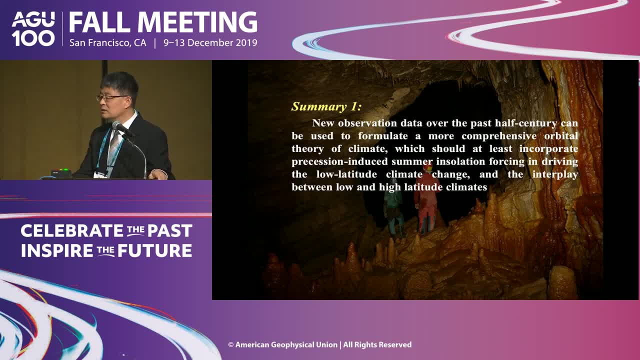 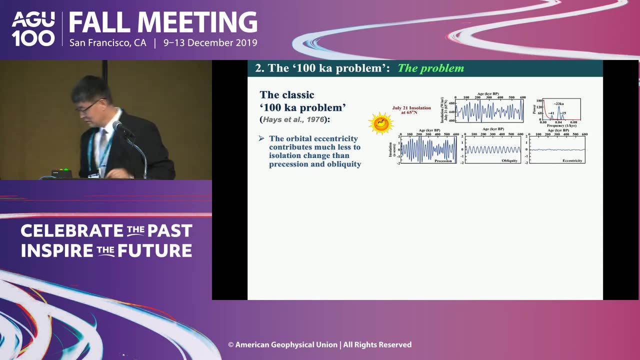 data may be used to formulate a more comprehensive orbitals theory of climate, which should at least incorporate precession-induced insolation forcing in driving, the low latitude, climate change and the interplay between low and high latitude climate. Okay, do I still have time? 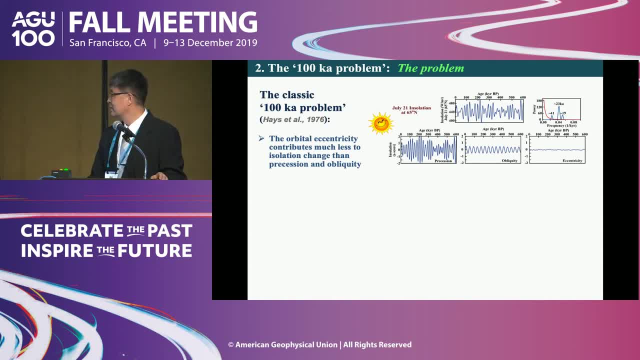 No, no, probably I can go through the second talk, but I have a little bit of time. Okay, I'm talking about a little bit about this 100,000 problem. The problem, as you probably knew better is really is this: 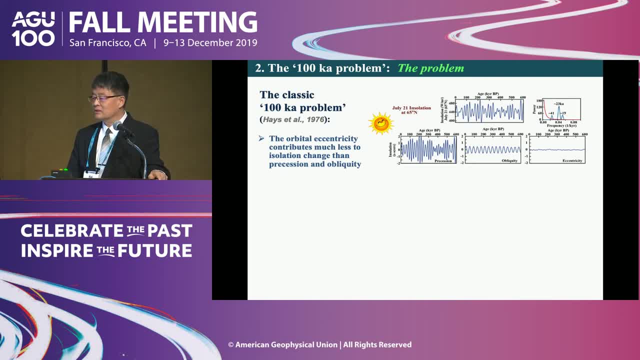 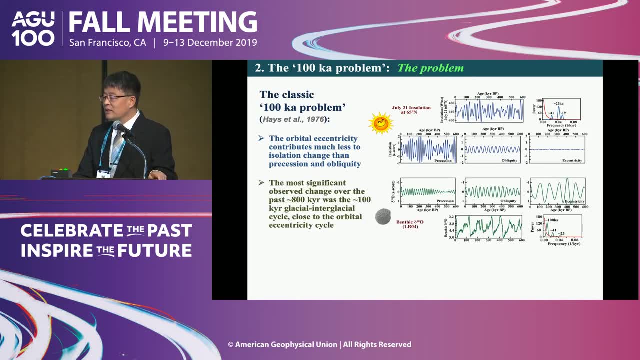 The orbital eccentricity contributes much less to insolation change than precession and obliquity. However, the most significant observed change over the past 800,000 years, over the past 800,000 years, over the past 800,000 years. 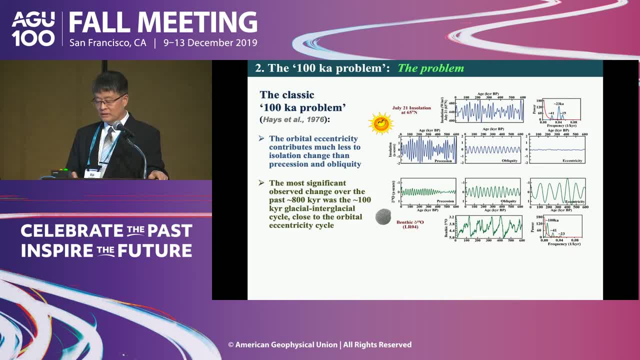 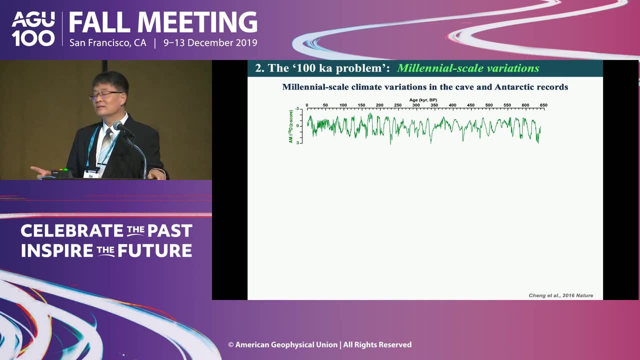 the interglacial cycle close to orbital eccentricity cycle. the interglacial cycle close to orbital eccentricity cycle. So there are a number of hypothesis there already trying to resolve this classical, longstanding issue. Here is our approach. This is the Asian monsoon record we mentioned before. 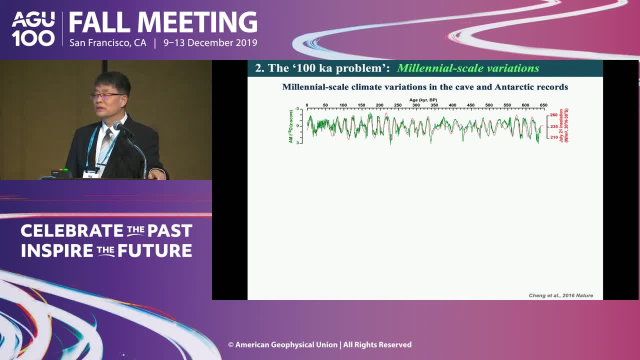 Then we knew that it follows some insolation closely. If we removed the insolation- always long-term, this kind of components- we get a residue. Well, I believe that the residue therefore characterize millennial scale climate variations. Here is the Delta D record from Antarctica: 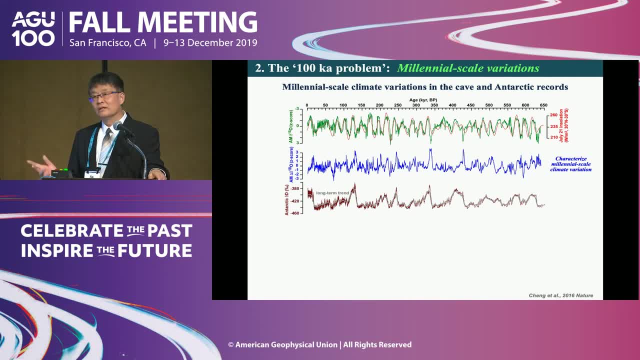 If you remove the long-term, mathematically long-term trend, or the long-term trend actually is the identical to benthic delta weighting record. therefore you get, Therefore you get another residue record. Therefore, we think this characterized. 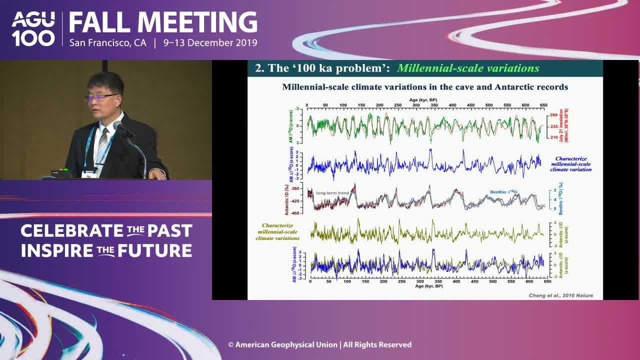 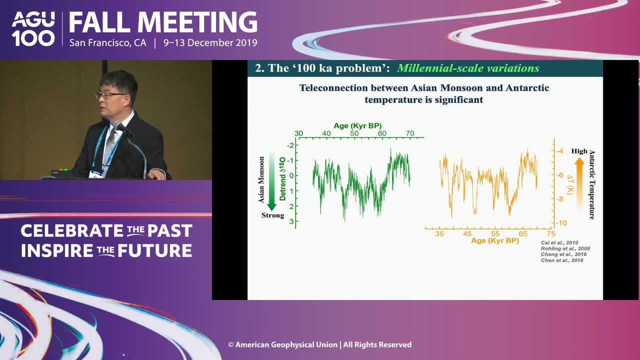 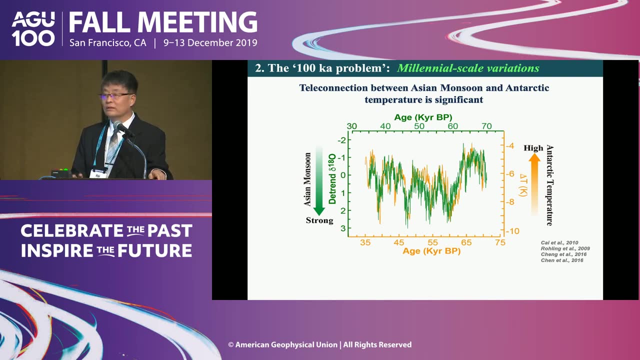 millennial scale climate variations. Those two records- they're virtually are just the same. So this is not surprising, because the teleconnection between Asian monsoon and Antarctica temperature is significant, For example. you can see, those two records can overlap during the last glacial period. 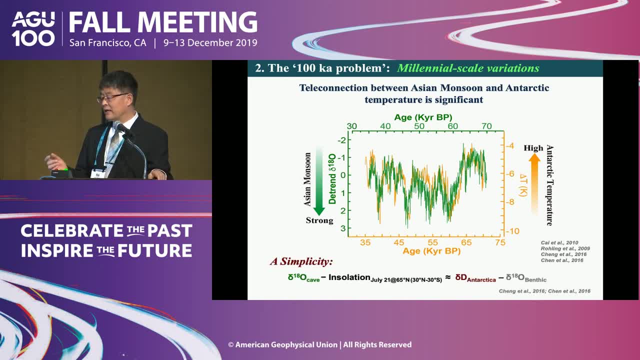 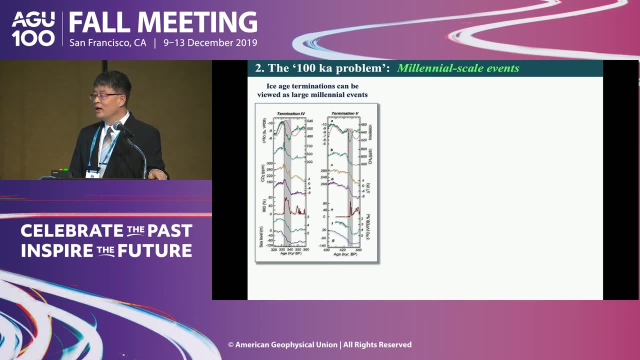 Then it demonstrate a simplicity. if you like delta weighting, a cave record. you remove the insolation component, you're gonna be equal to the Antarctic temperature. remove the delta weighting of benthic, So, on the other hand, ice age terminations. 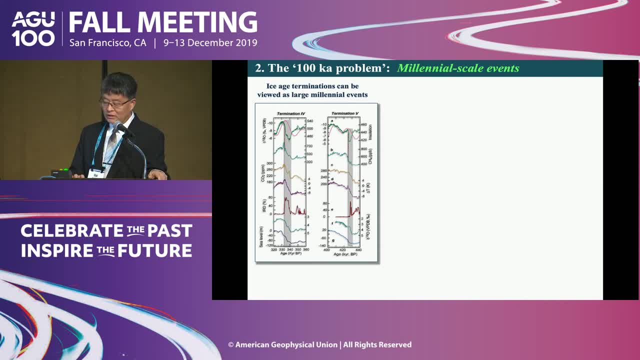 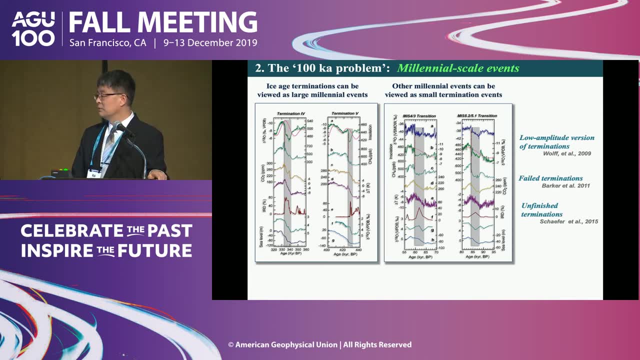 can be viewed as larger millennial events And other millennial events can be viewed as small termination events, For example, as people call it, whatever low amplitude version of the termination, or failed terminations, or unfinished terminations, Anyway, ice age termination events. 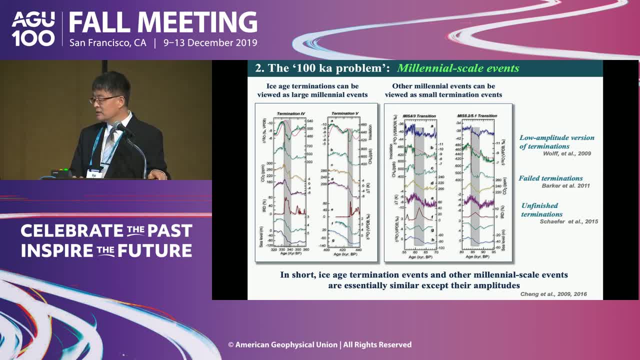 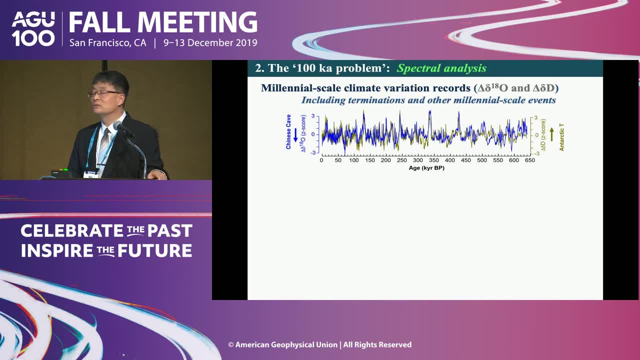 and other millennial scale events are essentially similar, except that they are amplitude. So now we think we have millennial scale climate variation records, those residue records, as I mentioned before, including terminations and other millennial scale events. If we do spectral analysis then we found that 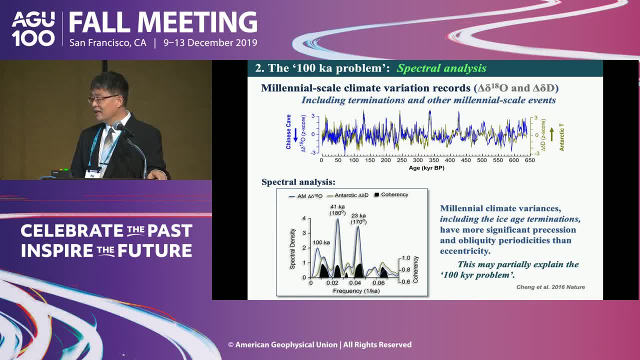 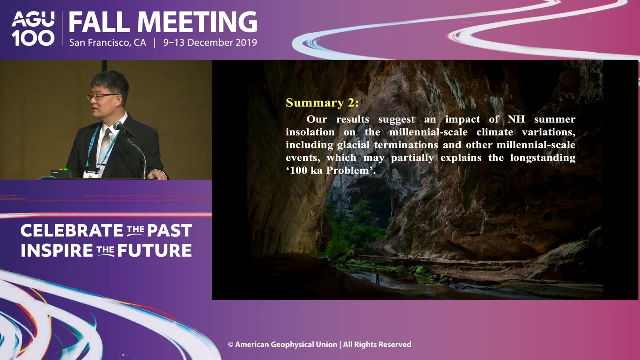 the millennial climate variations, including the ice age terminations, have more significant precession and obliquity periodicities than eccentricity. This, I think, may partially explain some aspect of 100,000 years problems. Here is the second summary. our results suggest an impact. 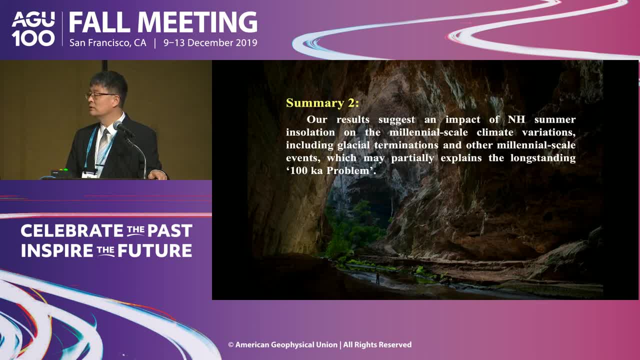 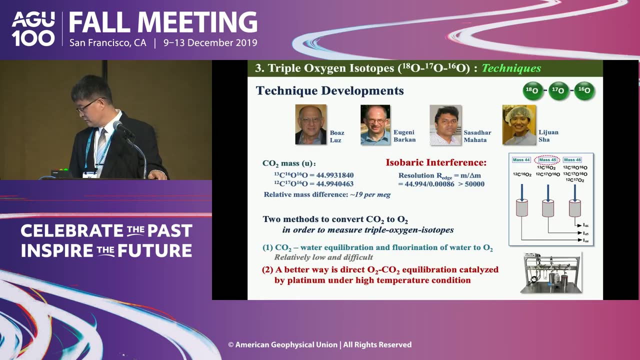 of northern hemisphere, summer insolation, millennial scale climate variations, including glacial terminations, and other millennial scale events which may partially explain the long-standing 100,000 years problem. If I have a few minutes, Oh still. 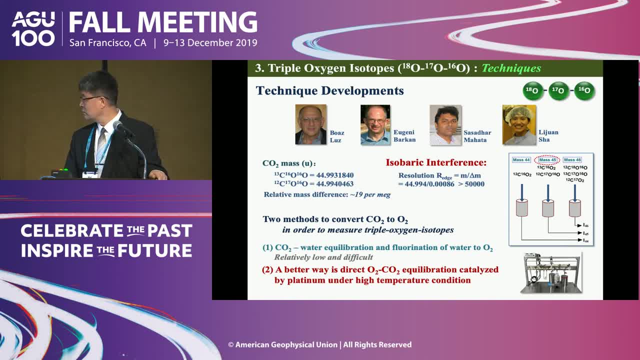 Plenty time. Oh, okay, 18 minutes are you talking about? That's too long. I thought it was total time is gonna be 50 minutes. Sorry about that. So therefore, the third topic is about recently progress in triple oxygen isotope. 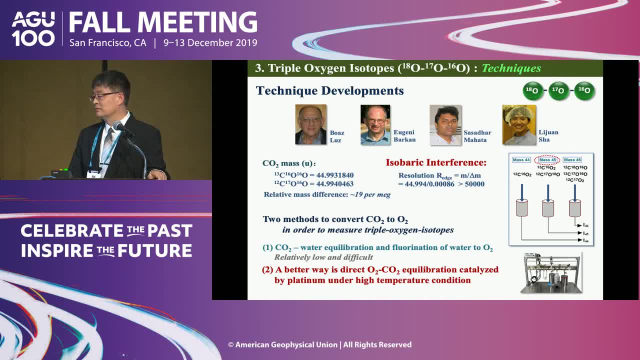 So technically there is a difficult because isobaric interference on the mass. 45, if you wanna measure CO2 directly, CO2, of course, is released from our carbon carbonate samples directly by the acid. Therefore we have to develop some method to convert CO2. 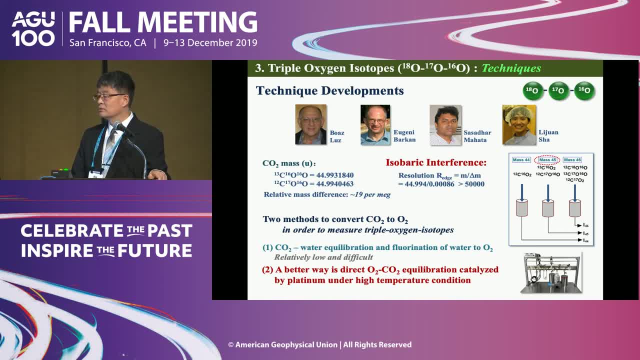 to O2, then measure O2 in order to measure triple oxygen isotope of the carbonate. So there are two way to do this conversion. We use the second way, which we think the here is the second way. we think that way is much better. 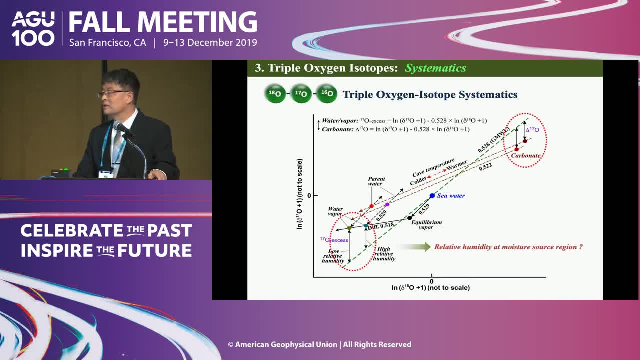 In terms of triple oxygen isotope systematics. I think we pretty much understand what's going on. This is our understanding. It's not that complicated but to be simplified essentially, basically, we would like to measure carbonate delta, 17 O excess. 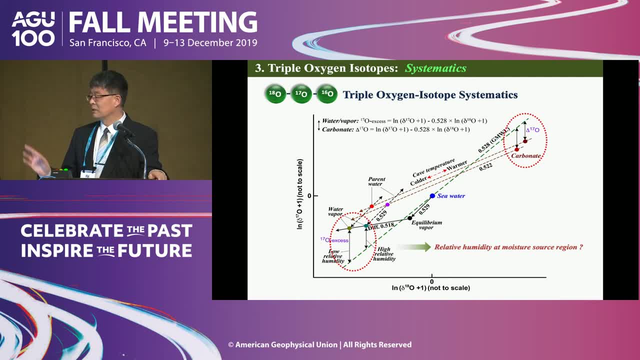 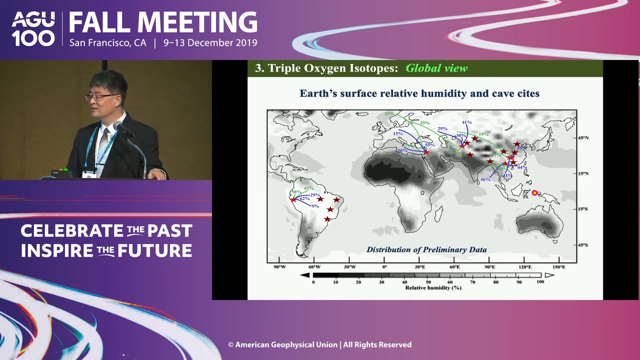 Therefore this notation is a little bit funny but because the conventional problem. Therefore we can get the information of the rainfall, delta 17 O excess, which then we can use to get the relative humidity at the moisture source regions. So here is Earth's surface relative humidity and cave size. 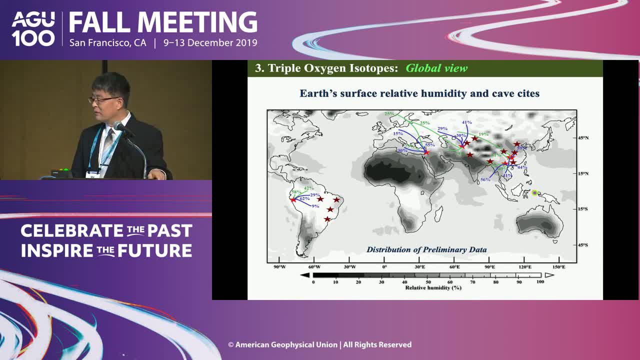 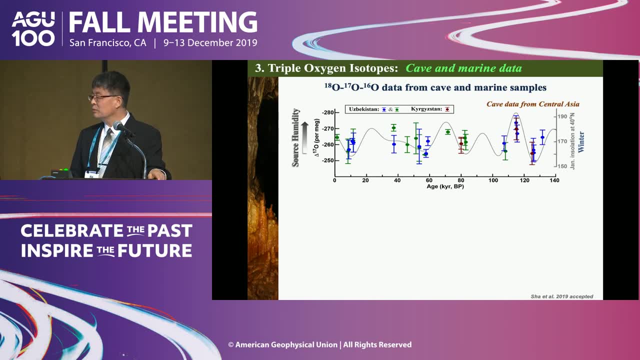 We already have some kind of a preliminary data from those cave size already. Also, you can see some example of the data. For example, the cave data from Central Asia show that it looks like it's for the winter installation in the winter precipitation. okay, 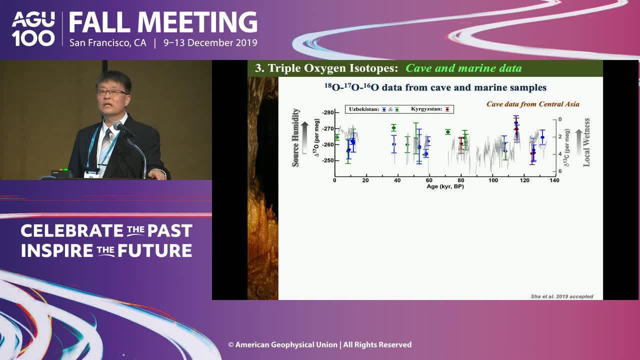 The regime. okay, There are also themes. There are some correlations with the local wetness. All that is seven. We also have a little bit of marine data from West Pacific warm pool. It looks like the data follows local summer insulation and have little bit of correlation. 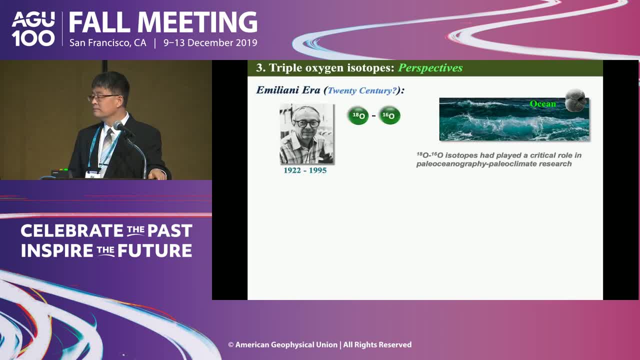 with the summer monsoon variations as well. So overall, in Amignani era the 18-0, 16-0 ratio of isotopes indeed had played a critical role in paleo-oceanography and paleoclimate research. 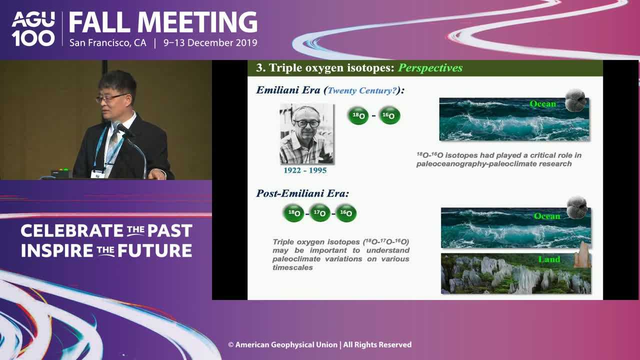 In the future. I think the triple oxygen isotopes may be important to understand paleoclimate variations on the various time scales. Now we are at the stage to have a big picture about the 17-0 axis in a global scale. So just like 1955, when Amignani published his 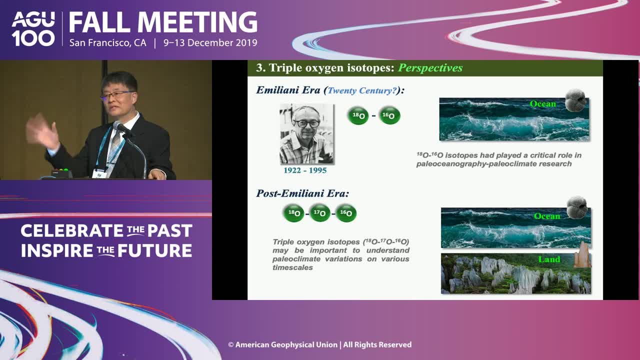 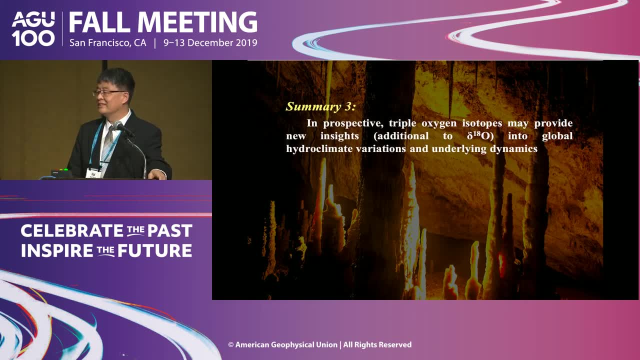 big. first like to first order what's the glacial interglacial cycle might be looks like. So here is the third, this summary. I think in prospective, triple oxygen isotopes may provide new insights into global hydroclimate variations and underlying dynamics. 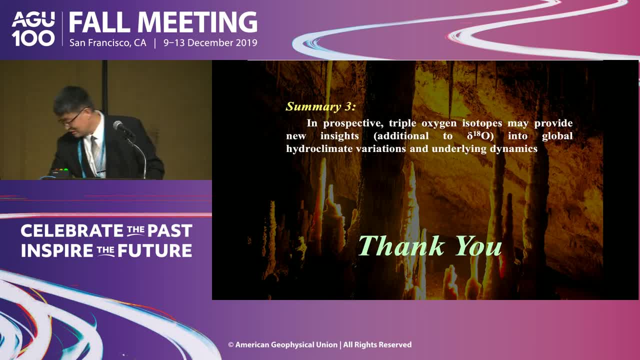 Okay, thank you for your time. So, before I open up to questions, I would like to present Hai with his fancy certificate from AGU, Thank you, Thank you so much. So questions: Yes, I'll ask it. Yes, 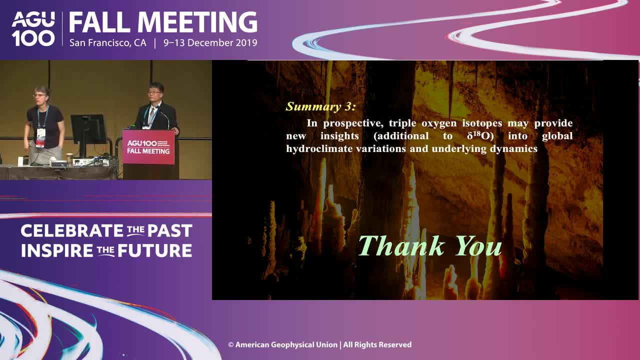 At first you were calling. Can you say one more thing? Yes, So how did you figure out what you could do about this problem? Okay, One hundred K problem, as I mentioned, is because the insulation it's tied to the initial, the Milakovich theory. 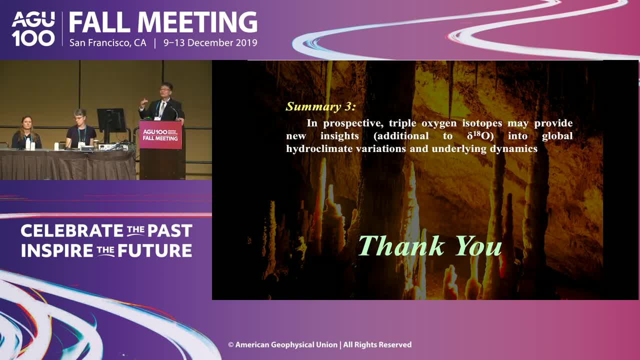 This Milakovich theory is standard summer insulation at the like the 65 degree is the main driver of the ice sheet change. then the ice sheet change affect the global climate. Basically, the main idea is this. Therefore, the Paleoceanographic evidence. 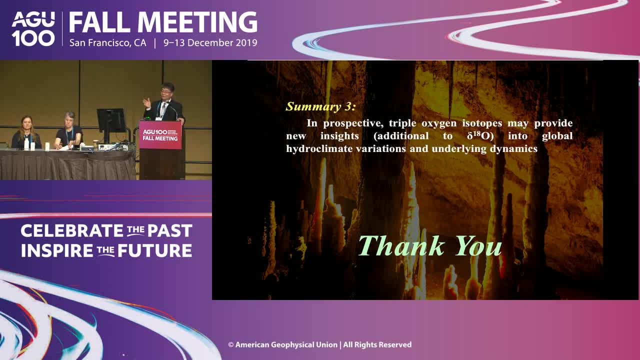 show that in terms of periodicity they match melancholy cycles like precession of liquid eccentricity. But, as I said, the contribution to the insulation change is mainly from precession cycles and obliquity cycles, not eccentricity cycles But the evidence from marine or delta weighting. 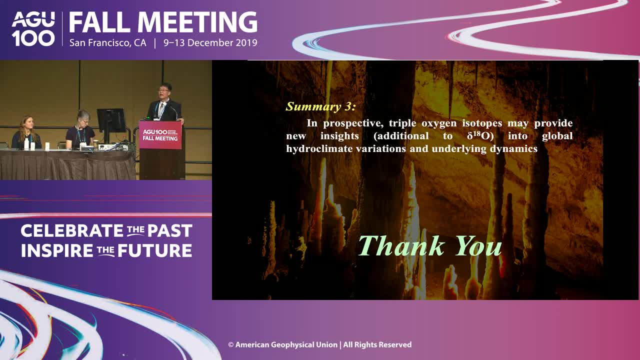 is actually the largest amplitude is 100,000 years. about 100,000 years cycle, not as predicted as the insulation cycle, which is dominated by precession and obliquity. So this is the problem itself. Then it's still the problem until now. 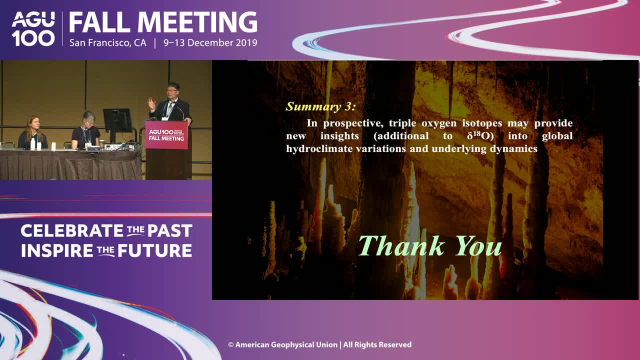 but I think if you just take the isolation, the ice age termination and the other millennial variability, ice termination is a millennial variability like several thousand years termination really fast. So therefore, if you do static tickets or this analysis, you're gonna see the main. 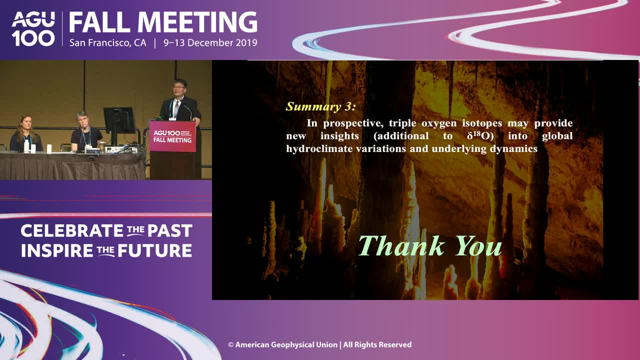 periodicity is not precession, it's indeed not eccentricity, it's indeed precession and obliquity. That means the long-term or the ice age. this 100,000 years problem is more or less not the insulation course. 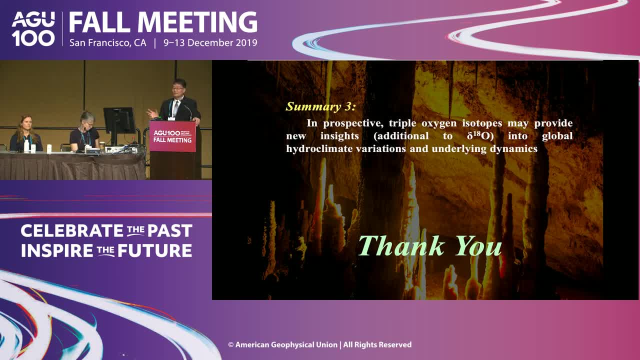 it's. possibly it's just internal. this ice sheet dynamic decided, contributed to the 100,000 years problem. This is our view on this issue. so What changed 800,000 years ago? That's also a good question. 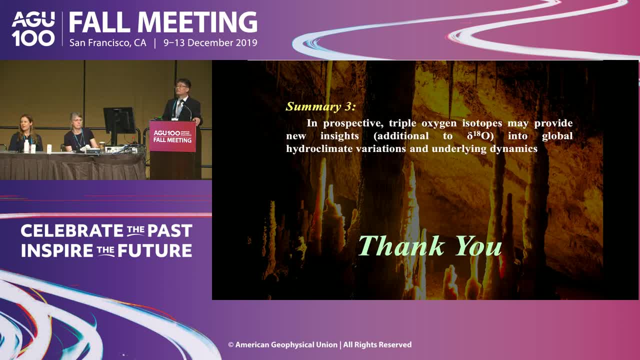 I personally think we do have some kind of split in record further back to 1.5 million years now, but not published yet. but to our record we still see the precession cycles dominant. but the marine record, you know that. 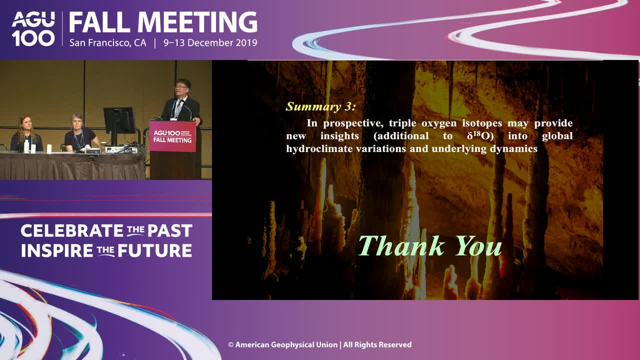 it's a 40K award, right, The 40K. it's sort of like. I personally don't think the precession dominant, that this precession is still dominant, because the same reason that just the ice sheet or temperature boundary condition are slightly different, 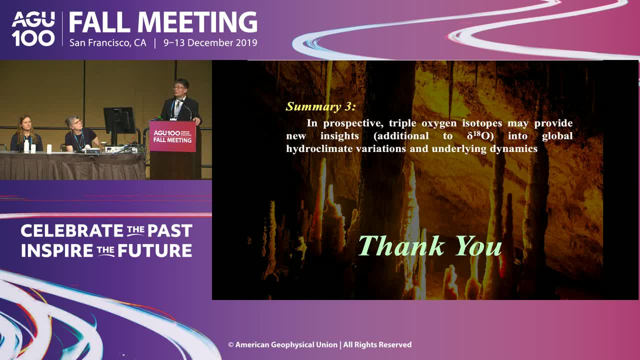 therefore, the internal ice sheet dynamics is slightly different. Therefore, everything is consistent. This is one of the reasons why the so we're not sure that, but we were finding that there are some accepted, so this was same. this is. 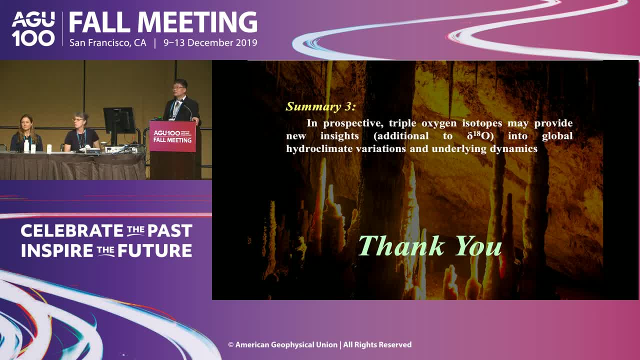 a very common issue, in particular for this market. I've also seen a lot of research, more public information about the Arctic ice sheet and, which is also a concern to the public, about the Arctic ice sheet and the what really could be done about it. 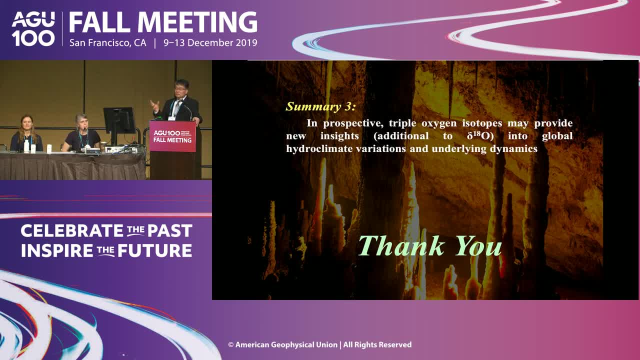 So what's your opinion about the Arctic ice sheet? There's a lot of things we've talked about, but this is, you know, this is a long standing issue. For example, the marine record is not really match the land record, for example, 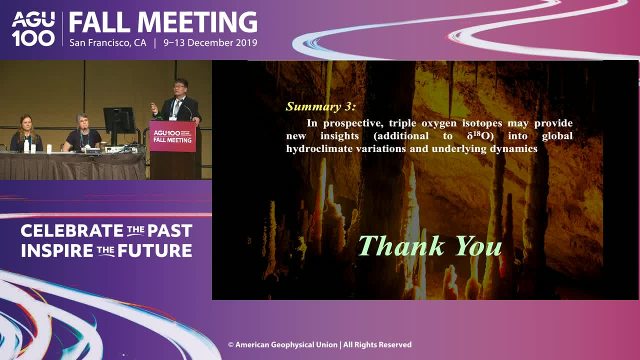 cave record and urban sea record. There are some fundamental discrepancy there. For Indian monsoon we do have long-term record which really match Eastern Asian monsoon nicely, but there's a difference. There is a slightly larger component, or periodicity is slightly more significant. 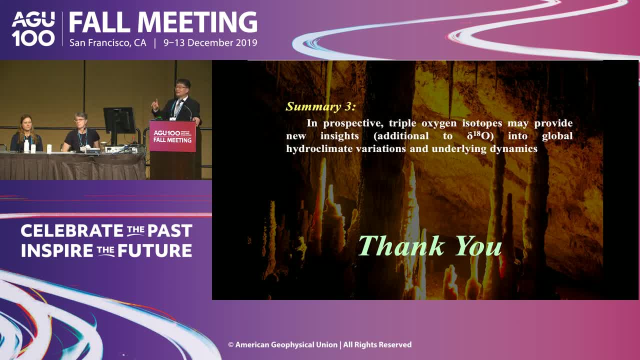 in Indian monsoon record. That's because I think I probably don't have enough time to explain why Eastern Asian monsoon has less interglacial cycle but Indian monsoon do have some interglacial cycles there inside of the Indian monsoon. 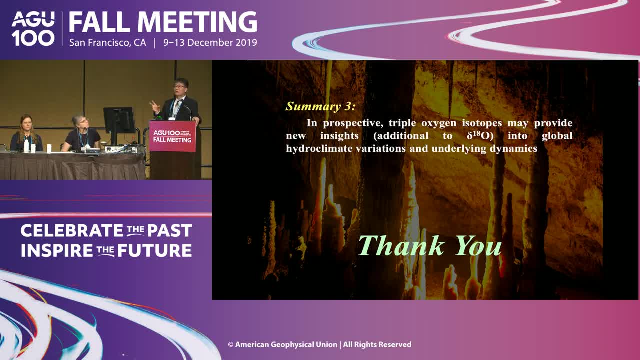 So in our East Asian monsoon record it's just a pure precession signal, but Indian monsoon has some- maybe 100,000 year cycle there. So the difference is that we recently understood what happened In East Asian monsoon: there is glacial. 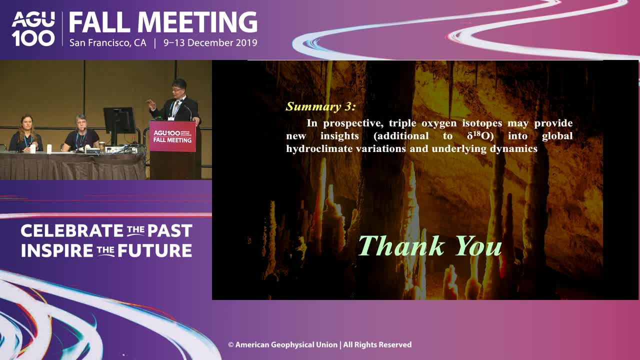 interglacial sea level components there, So that interglacial component canceled the influence from the interglacial impact But Indian monsoon doesn't. this is because continental shelf is very just extend really long distance during the glacial time because the sea level was low. 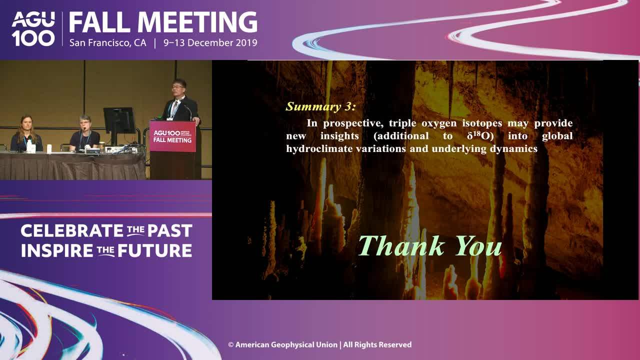 Therefore the source is far away. It could be like 1,000 kilometers away, the marine source for the East Asian monsoon, But the Indian side they're totally different. Therefore, this effect canceled the interglacial glacial cycle in East Asian monsoon. data waiting record. 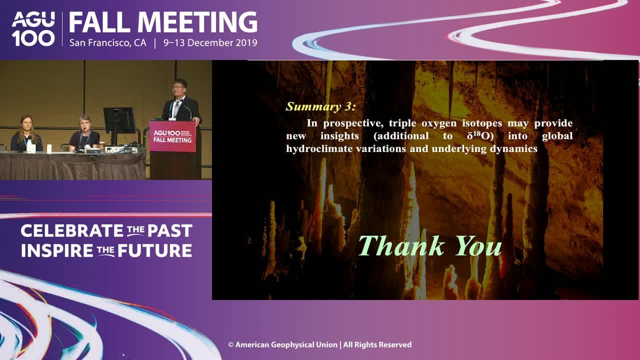 Because the source, the distance affected data waiting, But we did see this data waiting difference in terms of the, for example, the glacial, interglacial. this amplitude in Indian monsoon is like eight per mil, But in East Asia it's only four per mil. 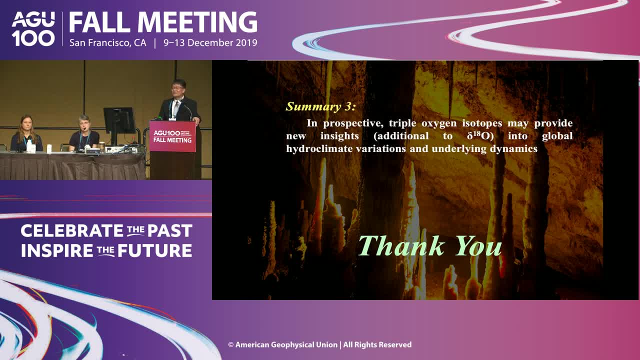 So other four per mil is just because cancer, right? That's why we didn't see It's the 100,000 years cycle. This is our story. Thank you for the talk. I just got one question. So we've used a lot of delta O18,. 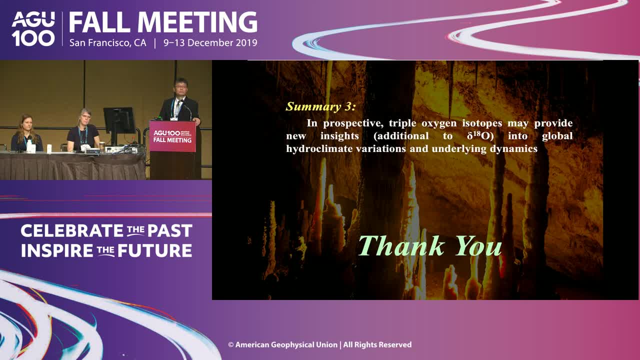 oxygen isotopes and also carbon isotope, of course. I just wonder if there's any chance we could talk about any use of calcium isotopes in speleothems and what they could tell us, if they can tell anything. You mean carbon isotopes. 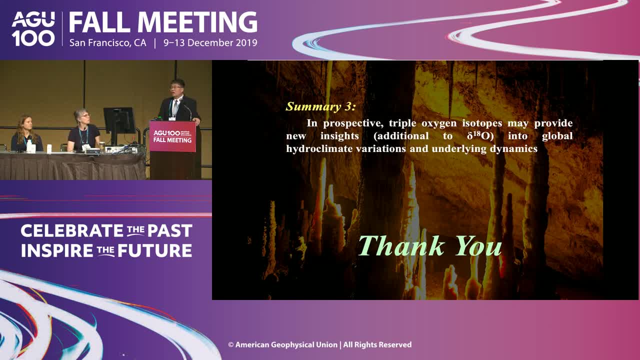 Calcium isotopes, calcium, Oh, calcium, Yeah, do they tell anything? Well, calcium, I think this is quite. I think I saw a few papers there, right, And it's not that exciting to me, probably. Otherwise, I will do that because we have the capacity.